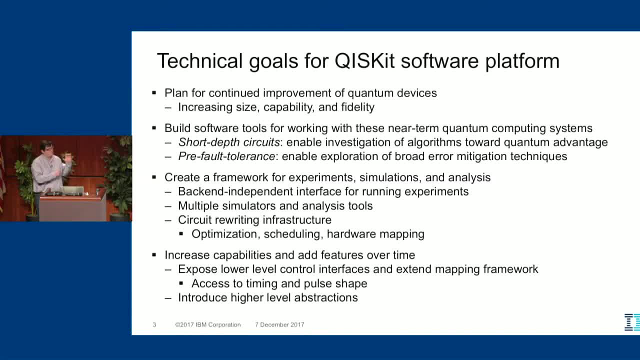 errors that we see in these systems. So we need a framework so that we can conduct experiments, can run simulations and we can analyze the data that we get back. We'd like this interface to be independent of the back ends, because again we're going to see new back ends in. 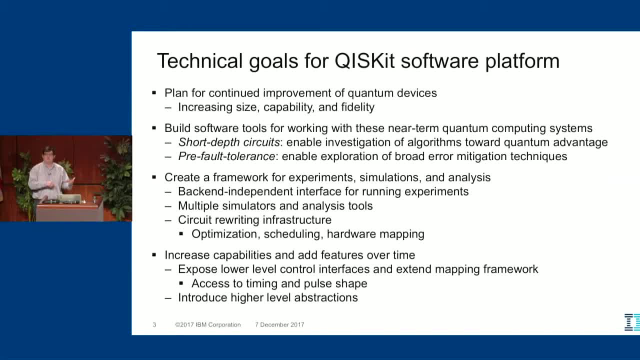 the future. We're going to see new simulation methods, We're going to see new ways of analyzing the results, So we'd like to be able to grow into that. We'd also like to create an infrastructure for rewriting the algorithms that we send the circuits And, at the very least, you know. 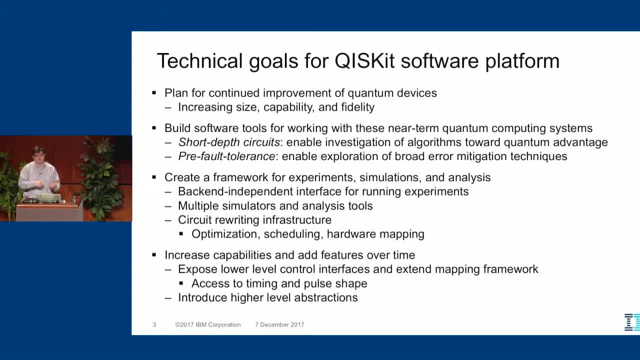 if this is meant to be back-end independent, we need to take the algorithms and schedule them and map them onto the hardware that we have. So we need an infrastructure for that and we plan to include that And then, over time, from where we are now to where we plan. 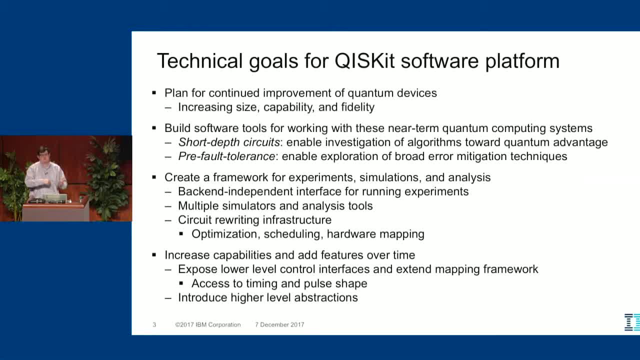 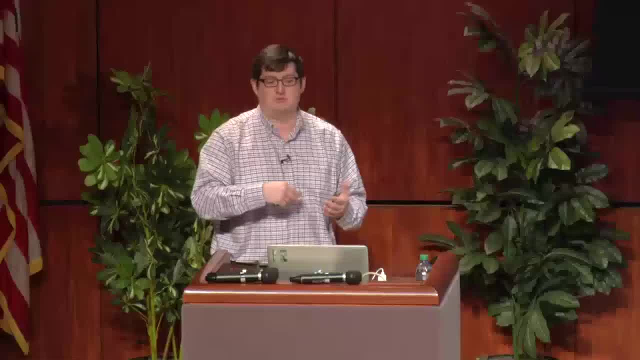 to go in the coming years. we'd like to expose lower-level control interfaces so that you have more control over pulse timing, You have more control over the process of mapping onto the device, more control over the pulse shapes, And we'd like to also move in the other direction. 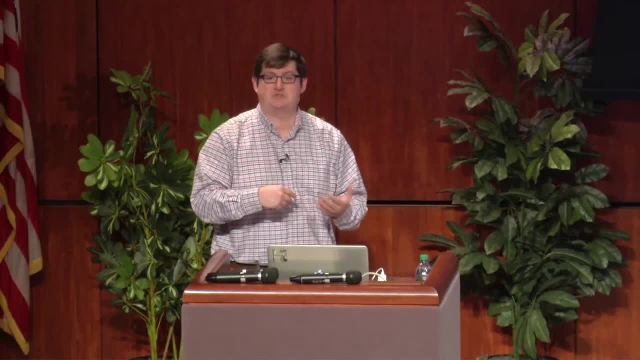 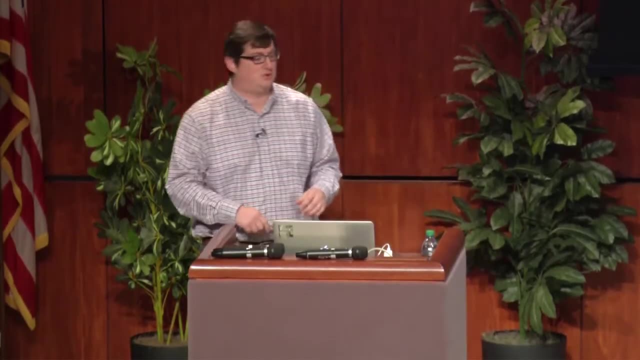 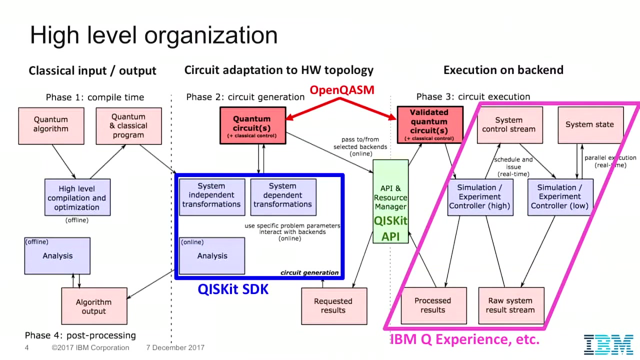 as well. so, expanding in both directions, introduce some higher-level abstraction so it's easier to program. All right, So as a touchstone for this whole talk, I'm just going to keep coming back to this, This block diagram. So what this is, this is you know, this is not exactly what's going. 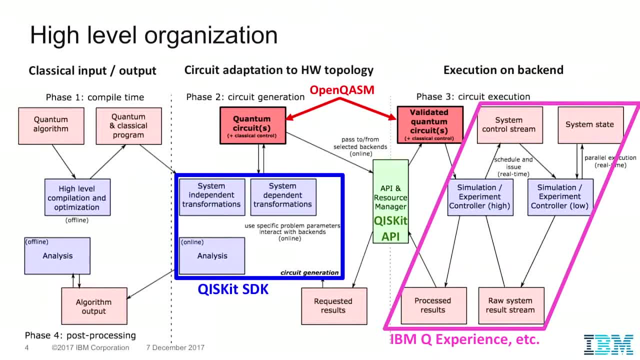 on, but it's a high-level organization of the pieces of the software as we would imagine them, And it's modeled after how you would think of a quantum compiler. Okay, But we're really going to focus on the right-hand side, the lower half of this process. All right, 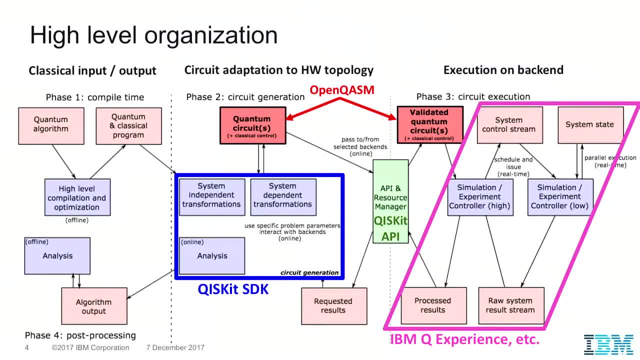 So, you know, on the left you have the quantum algorithm, You have some high-level description of it, You have the results you'd like to get And at some point you generate quantum circuits And these are stitched together by some kind of classical control. You know, at the moment, 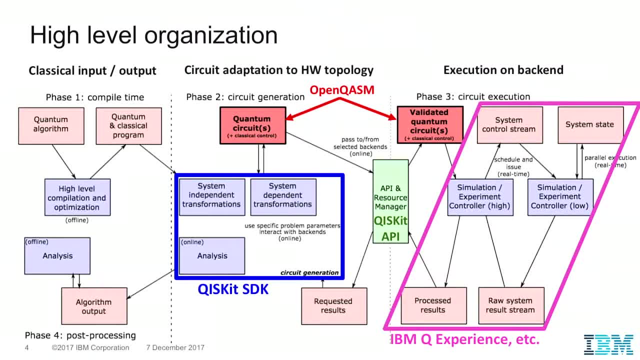 we have a limited set of classical control- I'll talk about that later- Right, But these quantum circuits are then transformed in some way and they are sent through an API On the back end on our systems. these are, you know, converted to pulse sequences. They run. 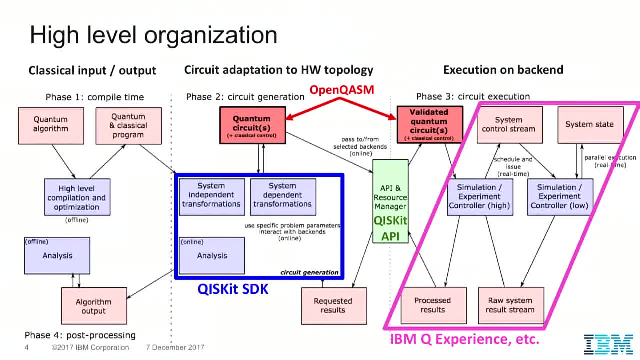 in the experiment. They're a set of controllers and whatnot, And these processed results come back through this API And you can request those results and then analyze them and then continue on. So, of these components, right, the quantum experience is everything behind this API. 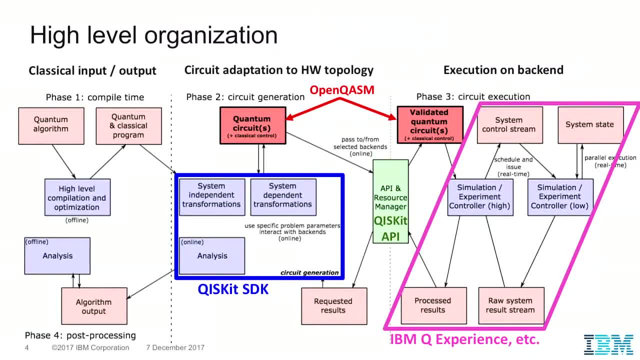 So the hardware, right now, you know the software that takes the circuits and maps them to pulse sequences, And then there's the API, There's our open interface language. This is something that will be familiar to people who have been in quantum computing. 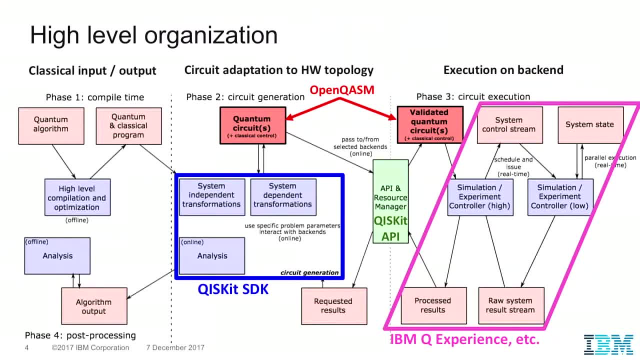 You know it's a list of gate operations that you can apply to our system And then this quiz kit software is built around the circuit abstraction so that you can write circuits and transform them and send them to the back end and process the results. 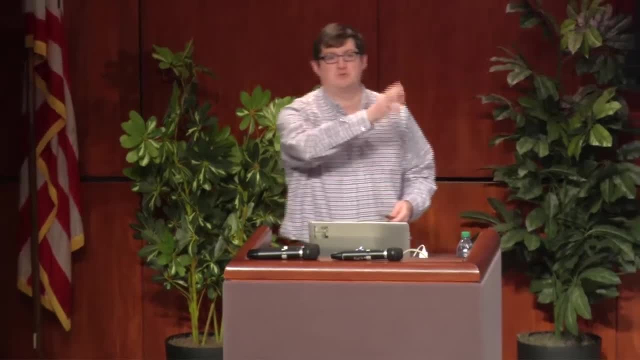 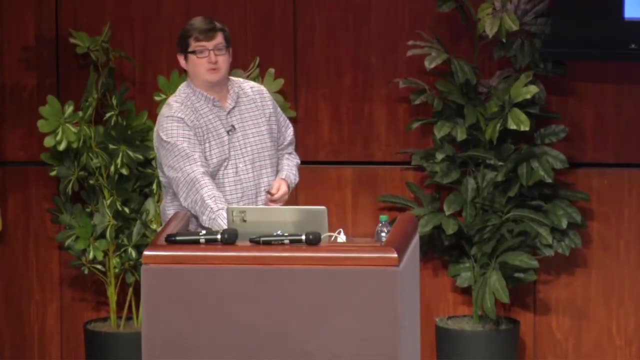 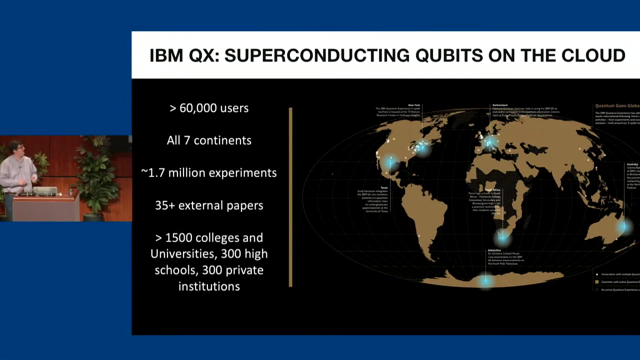 All right, So I'll keep coming back to this picture as we move through these pieces, And I'll start from the right and move to the left. OK, So I'll start with the quantum experience And so, just to say so, the quantum experience went online about a year and a half ago. 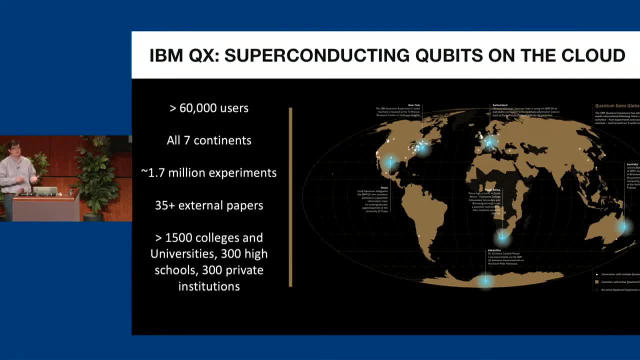 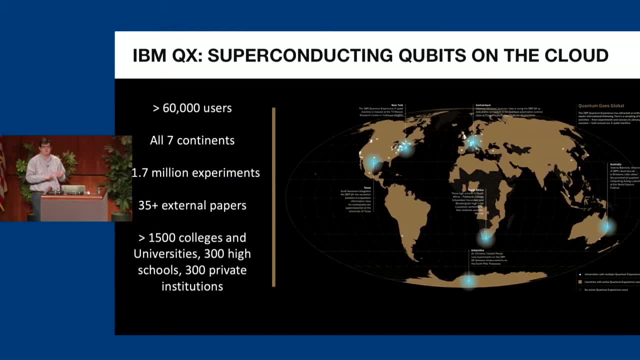 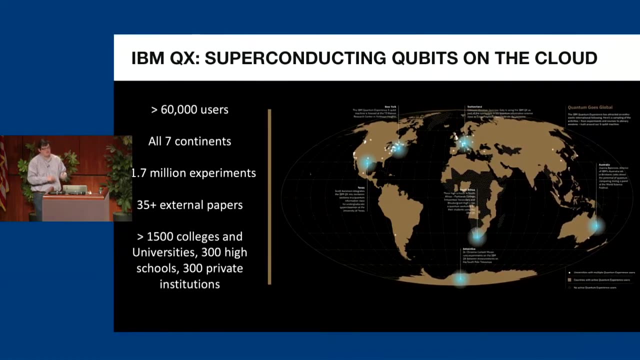 And in that time we now have more than 60,000 users registered. They've logged in from all seven continents, from many universities and colleges and learning institutions. People have run almost 2 million experiments on the devices that are there and have posted. 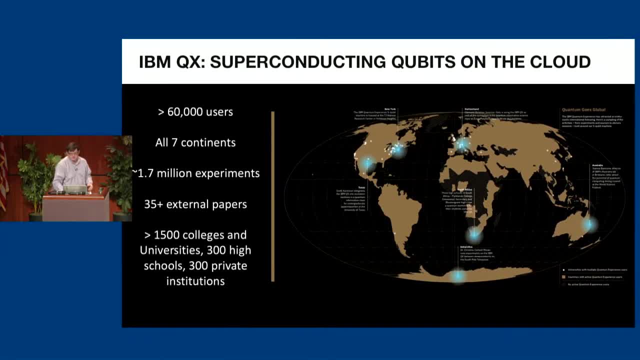 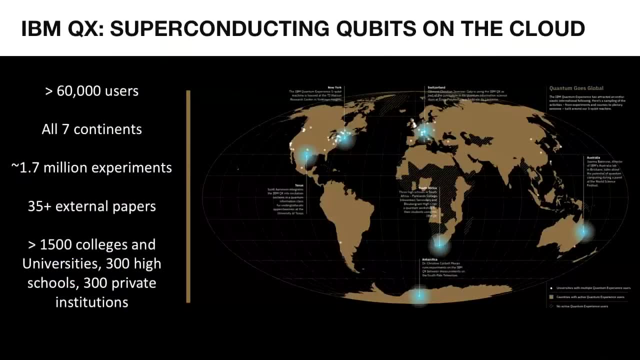 many papers to the archive as well, investigating the system and what it can do. For example, and just to explain what's in this picture, right, These highlighted regions are regions where people have logged in and used. these are countries where people logged in and used the quantum experience. 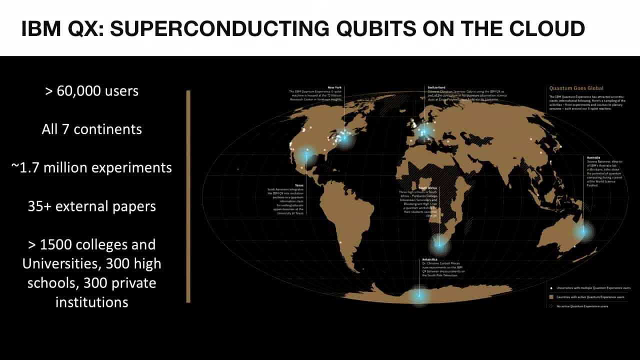 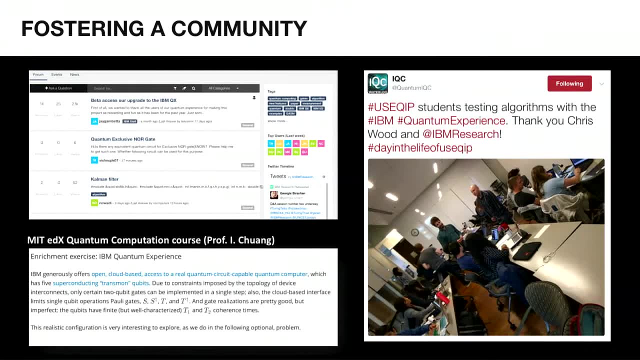 And the dots, I think, are learning institutions, educational institutions. So, as part of the quantum experience we've been trying to create, trying to engage with the broader community of educators, developers, students, Researchers Who are interested in using quantum. 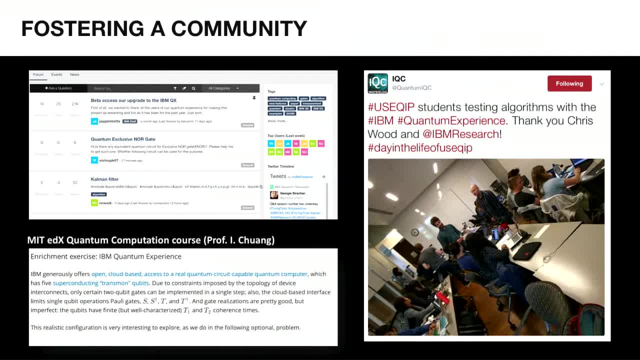 Why it feeds them in using these devices and learning from them. So we've been traveling and engaging with students. This is an example at USQIP. at the Institute for Quantum Computing, Chris Wood is working with students to run examples on the quantum experience. 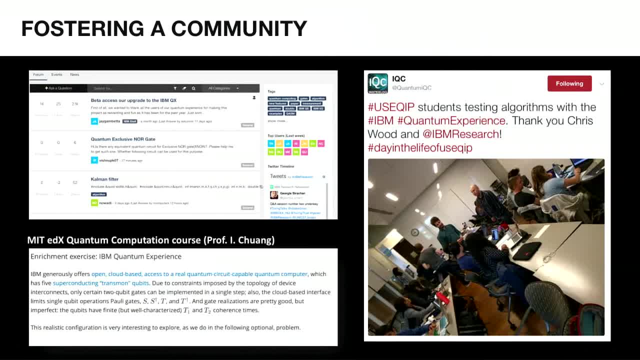 This is a community, like a forum that's available on the quantum experience website, where people from the public who've requested accounts and researchers- I mean everyone- can ask questions and answer each other's questions, And we also do our best to moderate. 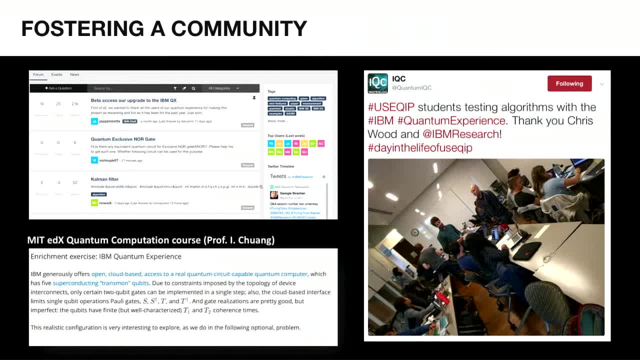 and answer questions that come up as well. And here's an example from, I believe from last year on the MIT edX quantum computing course run by Ike Chuang, where one of the extra credit exercises was to go and look at mapping circuits. 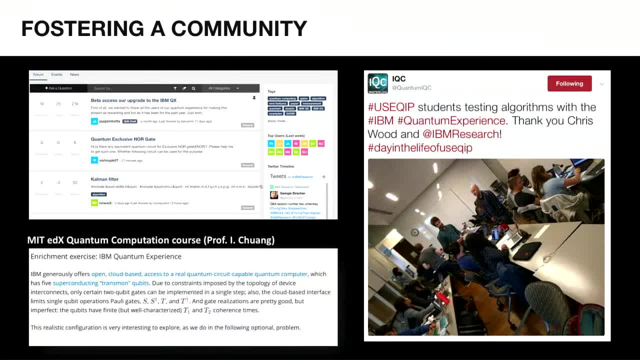 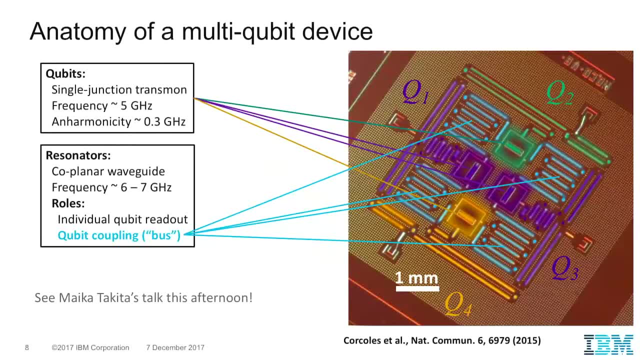 onto the quantum experience, the 5-qubit device. All right, so I'd like to say a little bit about what the hardware is that you're controlling I'm only going to talk about, I'm just going to highlight a few things. 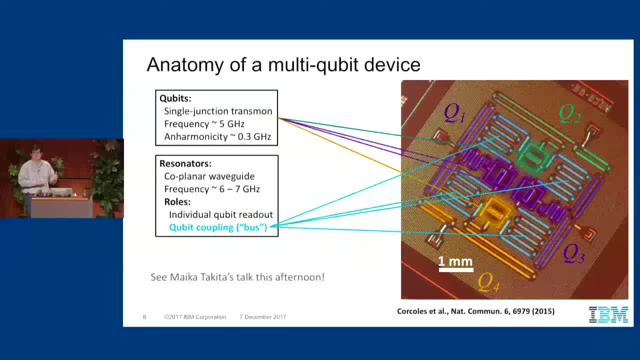 If you want more detail, definitely come to Mike Atakadu's talk this afternoon or at one of the breaks corner an experimentalist and ask them questions. So what you see here is this is a 4-qubit device And in these pockets are these single junction transmon qubits. 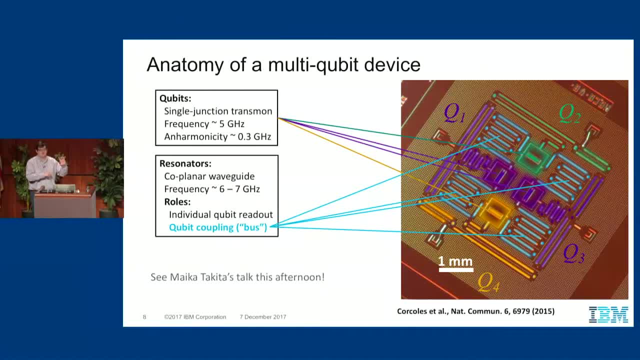 And just to give you an idea, right, the qubit transition is 5 gigahertz. The second excited state is slightly, you know, is offset by this anharmonicity. just to give you an idea of the kinds of parameters. 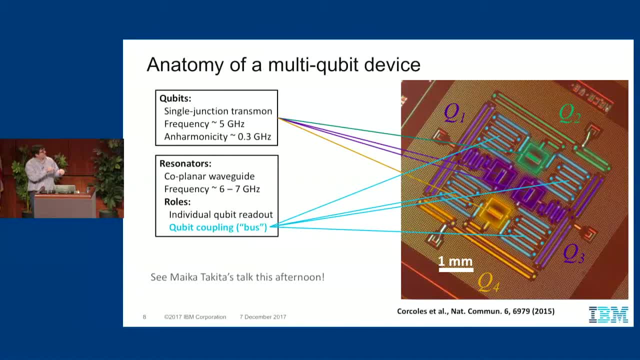 that are in these systems And these devices are coupled by Coplanar waveguides. So those are these blue and other colored features here. The blue is the you know, the blue is the you know, the blue is the you know, the blue is the blue. 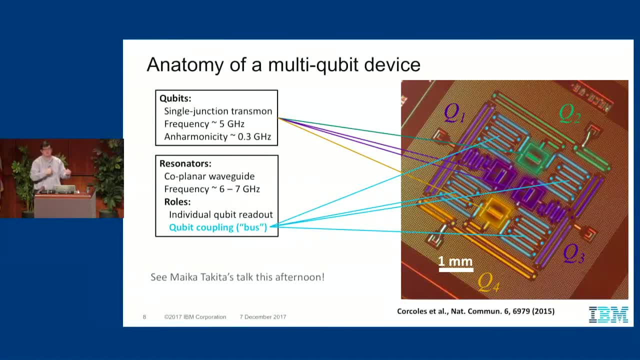 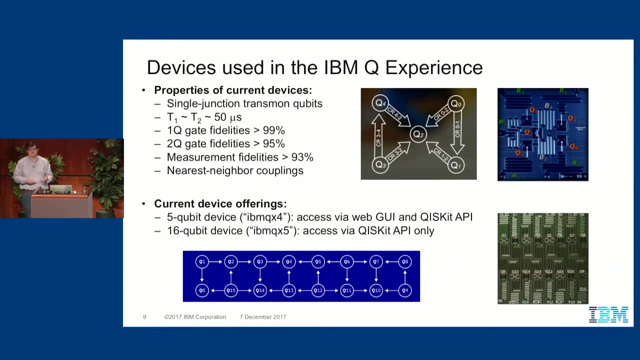 The blue resonators act as buses that couple neighboring qubits And the yellow act as input and output. you know readouts and drive lines, All right, so the devices that are used in the quantum experience, again, these are single junction transmon devices. 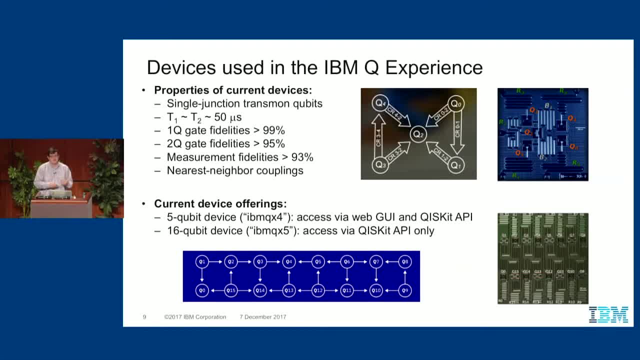 T1 and T2 are about comparable. They're about 50 microseconds In fact. you can see all of this if you go to the quantum experience and you look online at the interfaces. But these are the single qubit and two qubit gate fidelities around. 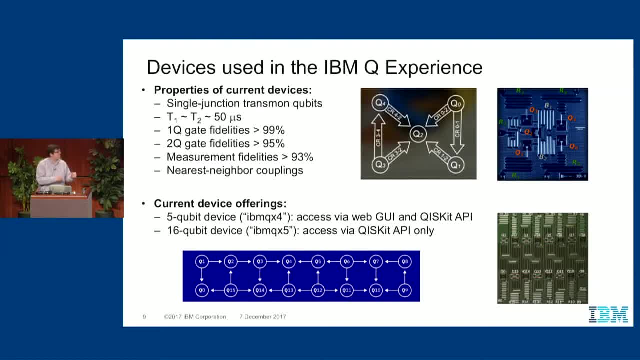 you know error around a percentile. You can see the error around a percent to five percent. You see the measurement fidelities And all the devices are some kind of planar geometry. So the five qubit device looks like this bow tie. 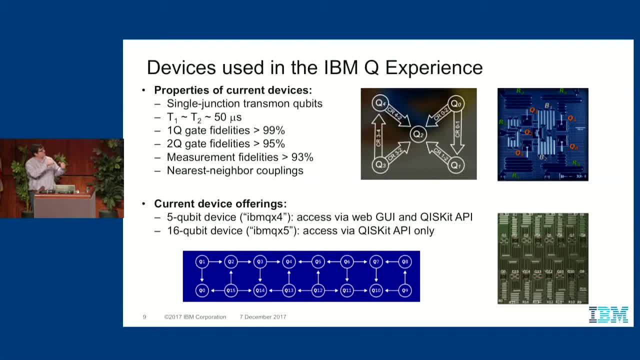 And these are the interactions that are available. And here's a picture of it. And this is the 16 qubit device. So it's a dual rail, two lines connected by edges. This is a picture of the device as well. So these are the five and 16.. 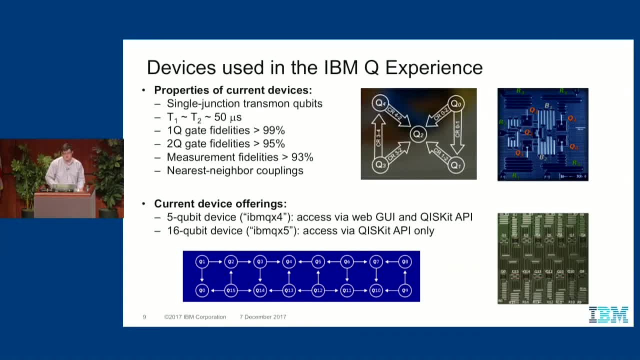 The five qubit device is available on the graphical interface And the 16 qubit device is available on the graphical interface And the 16 qubit device is available on the graphical interface And the 16, you can access through this software stack. 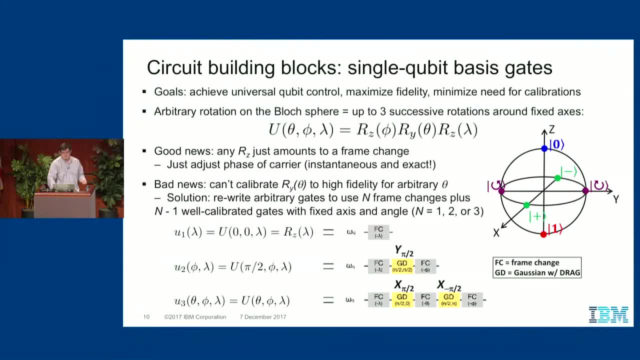 through the API. All right, So good, All right. So I'll just say a few more words about what the gates are in the system so that when we see them later, you know what I'm referring to. So we need single qubit. 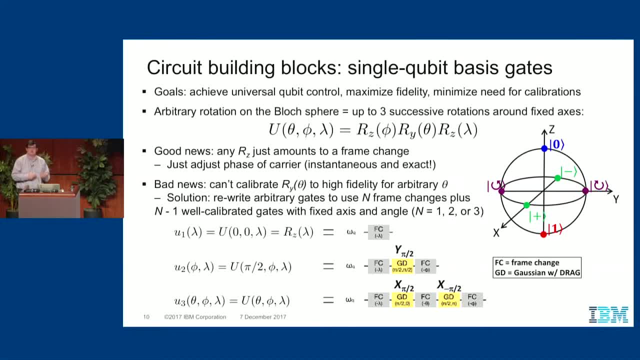 We'd like to have arbitrary single qubit gates and then some entangling gates so we can implement universal digital computation. And I mean here's how these are implemented. So generally, we want to apply something in SU2, some single qubit gate that's arbitrary. 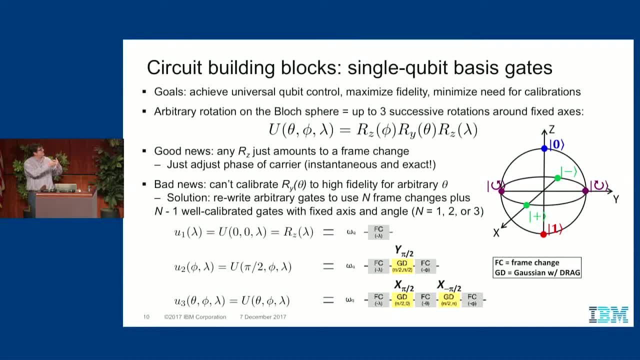 We decompose this into Euler angles, so ZYZ rotations Right. And it happens that these Z rotations are easy to apply by adjusting the phase of the carrier, So they are very accurate and fast. So it helps us to decompose The pulse sequence into something of the form. 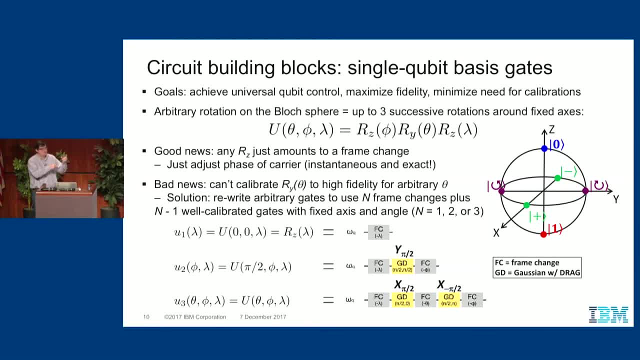 where we have this Z rotation and then we have some single calibrated gate that we apply in between these phase changes. So that's how these are implemented. If you just want a Z rotation, then you can apply this gate. that's instantaneous And there's no pulses, right? 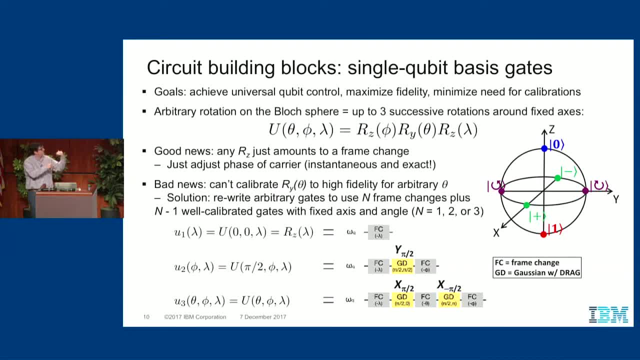 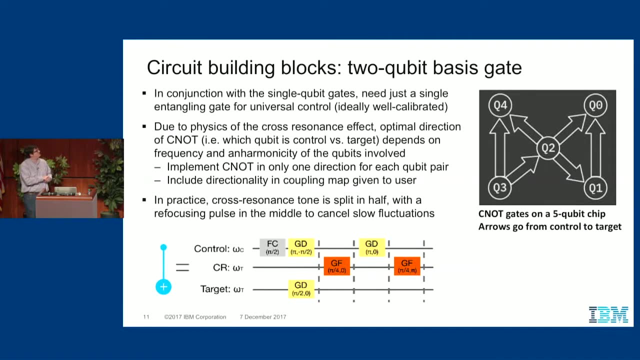 If you want to apply something that's a power 2 rotation, then you can apply this gate. That's one pulse. And then if you want to do something in general with two pulses, you can apply that. The two qubit gate is what's called a cross resonance gate. 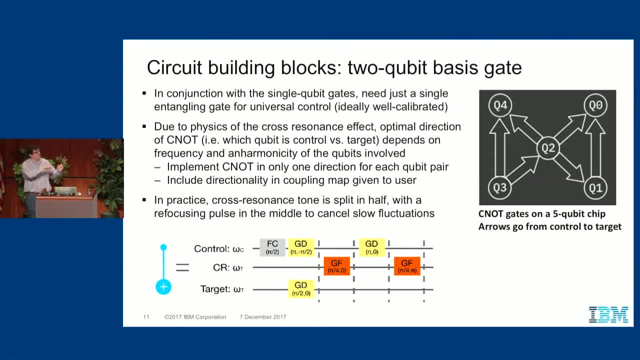 And for this talk, what's important about it is that it's directional. So there's a control qubit and a target qubit, And there's one direction where this gate is faster than the other. So that's why we do that this way. 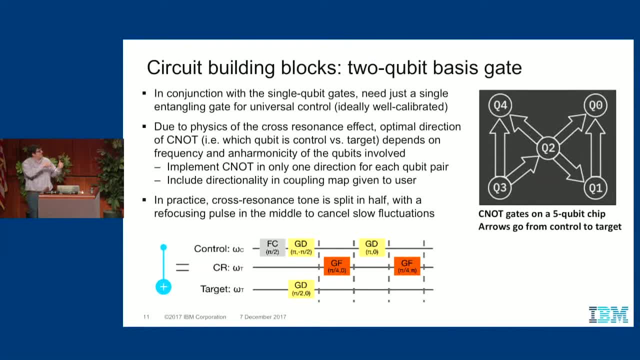 And in practice, if you're interested, this is implemented by a sequence of pulses that correct for some slow fluctuations. So this stands for this frame change, the Z rotation, This stands for a drag pulse And this stands for a flat top Gaussian pulse. 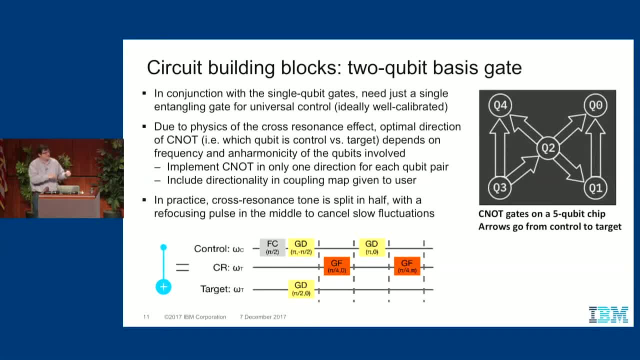 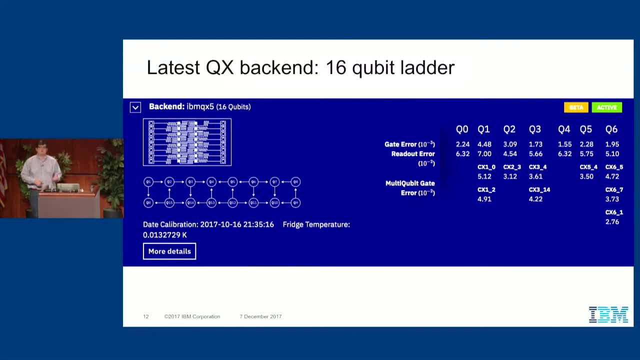 something that's stretched out. All right, So that gives you an idea of the 1 and 2 cubic gates in the system. All right, So if you go to the Quantum Experience website and you don't even have to log in, actually, 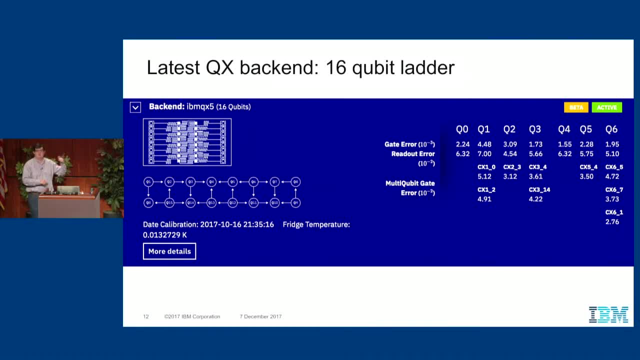 But if you look at the top, each of the back ends, the on-dis, Simone, the devices are, are listed there. this is the the latest back end in the sense of having a new topology, a new layout. all right, so this is the 16 qubit device. 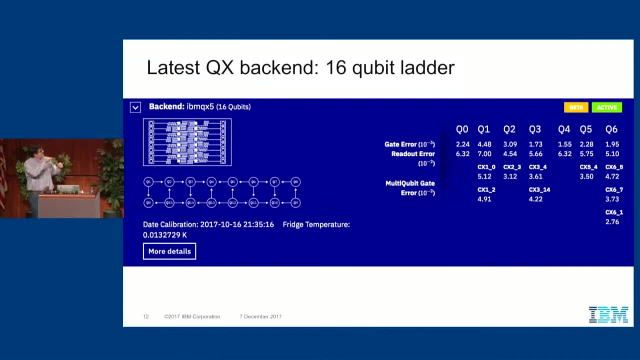 this is the, the picture of the mask. these are the. now you know, these are the CNOT directions and what you can also see is the last time, the caliber now. I grabbed this in right in October, but this is calibrated in the morning and evening, I believe. maybe it's calibrated once a day. anyway, you can see the latest. 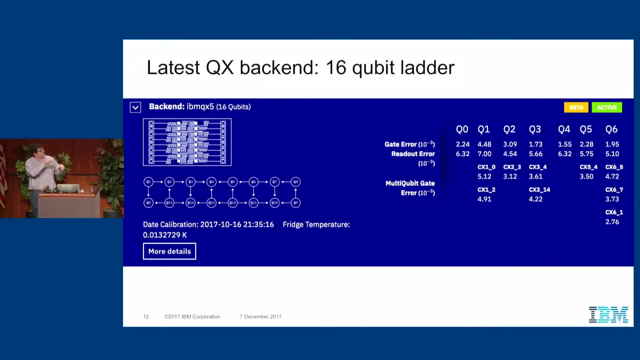 calibration there and then the results of that calibration is characterized by randomized benchmarking. so there's a single qubit gate error across here. this is cut off. there are 16 qubits readout error for each qubit and then the multi-qubit gate error. so these these numbers are consistent with what I said. 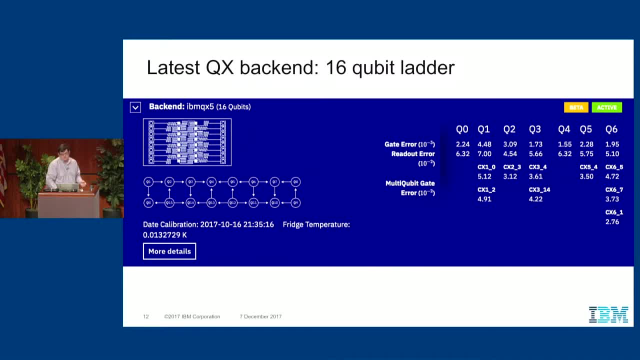 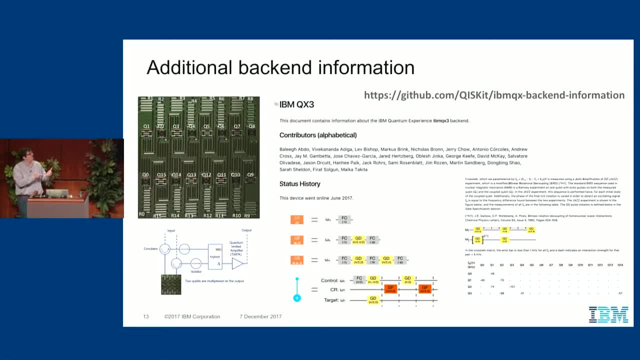 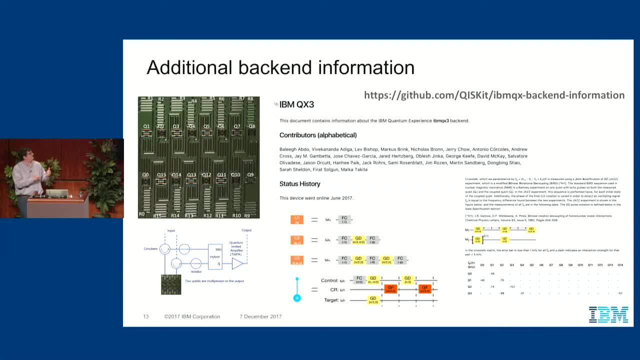 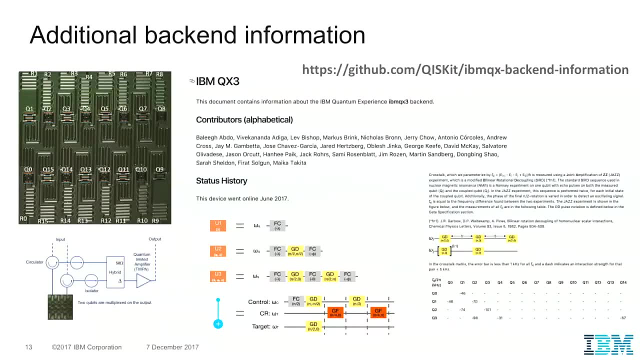 this URL and what you can find are you know? you can find each device. you can see, you know who's contributed to this device, its history, information about, say in this case, how the readouts are multiplexed, how the gates are implemented, and over here is an example of how the how the crosstalk is. 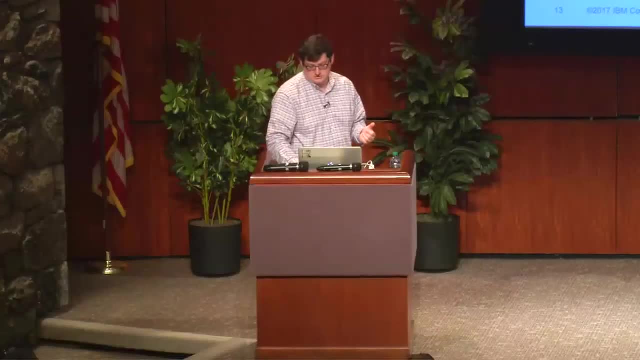 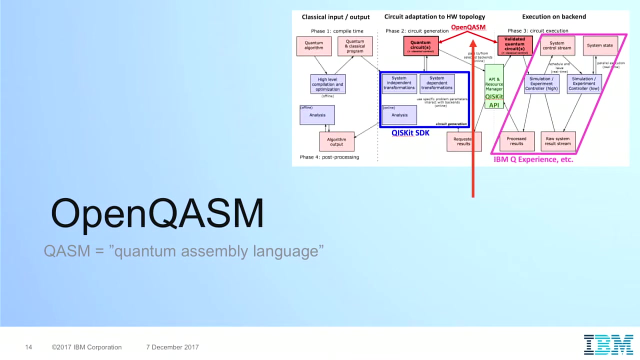 characterized in the device. okay, so please have a look at that if you're interested. all right, so those are the devices that are available in the quantum experience, and now we'd like to think about programming them. so we've chosen an intermediate representation of our circuits. that is, you know, it's based on a quantum. 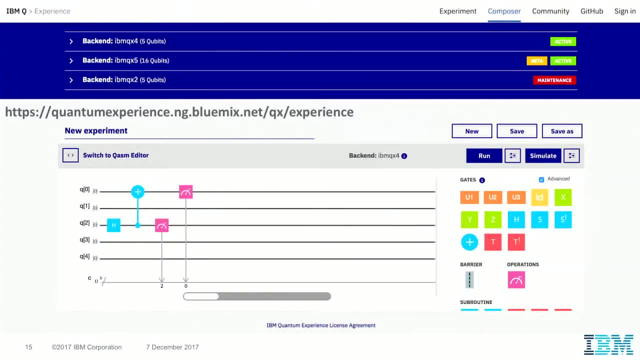 assembly language type description. this will be, I think, familiar to many people right this, the. the model is that you have some register or registers of qubits, you have some set of classical registers, and I'll say these just conceptually. these registers are somehow close to the. 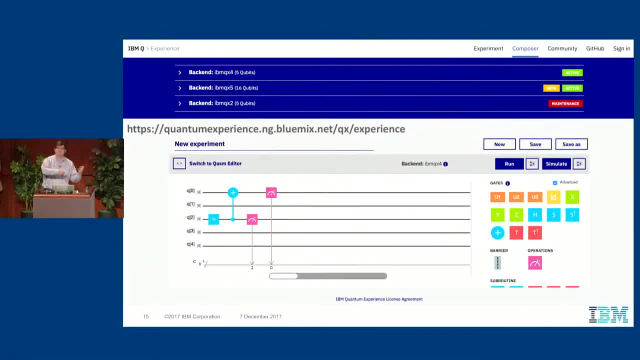 machine so that you can interact with them and feedback from them. eventually, that's what these aren't meant to represent: all the classical memory you're ever going to use in your quantum program. they're meant to represent something close. this is a picture, by the way, from the quantum experience from the 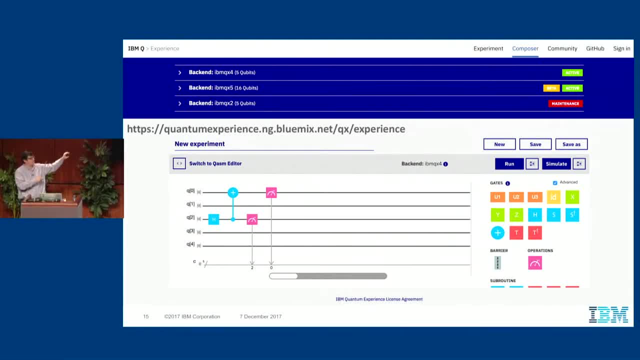 composer where you can take gates and drag and drop them and construct a circuit and then run it. so I'll just say, you know, here are the. these are these u1, u2, u3 gates, the single qubit gates, and this is the two-qubit gate and the rest of these are constructed from these or from doing. 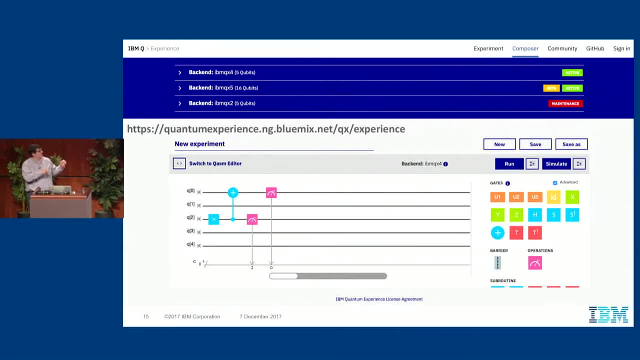 nothing. And there are some other instructions, for well, I'll come back to these later. right, There's a measurement and there's a way of controlling the timing. Okay, All right, so a little bit more detail, Since this is a tutorial. eventually, I'm going to 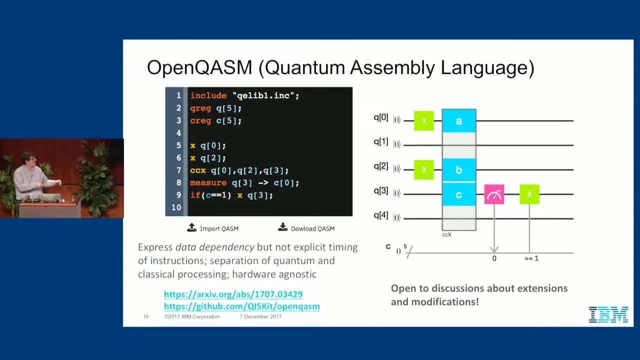 get to the point where I'm showing you lots of code, so we'll kind of start going in that direction. This is an example of a program that's written in OpenChasm, So it has these features right. It has quantum and classical registers, has some way of including definitions. 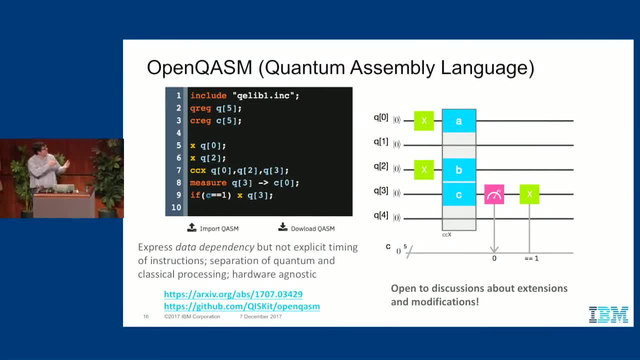 of gates, And then right, it's just instruction after instruction, together with what it acts on, And so there are a couple things that I can point out that are maybe interesting or different from other assembly languages. One is that it has a way of hierarchically- 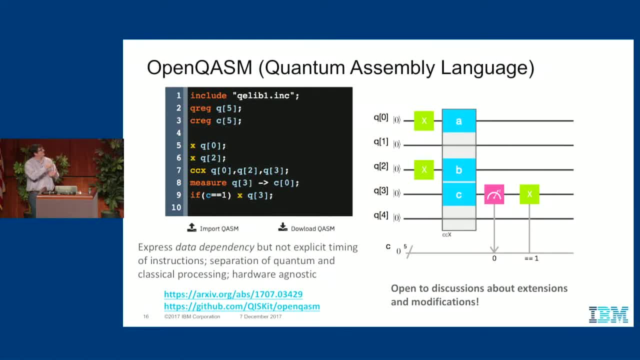 defining gates. So here's a Toffoli gate. It's defined in here, right, and it's put here, but that's constructed from you know C-naughts and Ts, as you'd expect, and those are constructed from Us. 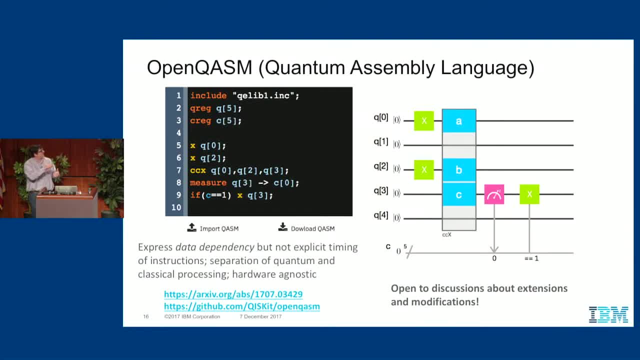 Right, And it has a mechanism for measurement and feedback. So measurement says where to put the result and then, based on the values of some register, you can apply operations afterwards. Okay, Now, at a high level. what this is meant to express is data dependency. 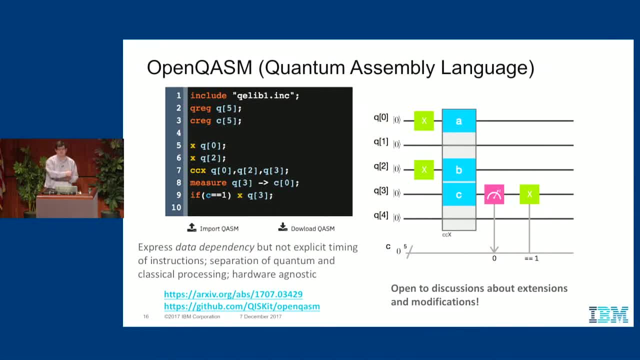 You know, do this, then do this, then do this, and here are the inputs I need to do the next step. There's no explicit timing here. The timing happens later, at a lower stage. Philosophically, we want to separate quantum and classical. 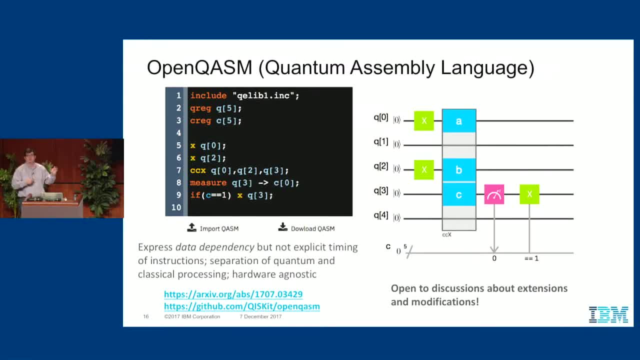 We want to separate quantum and classical processing as much as we can. This is meant to describe all the quantum computing, and the classical processing should be sort of encapsulated elsewhere. So right now, that's very simple. There's just this: if, but in. 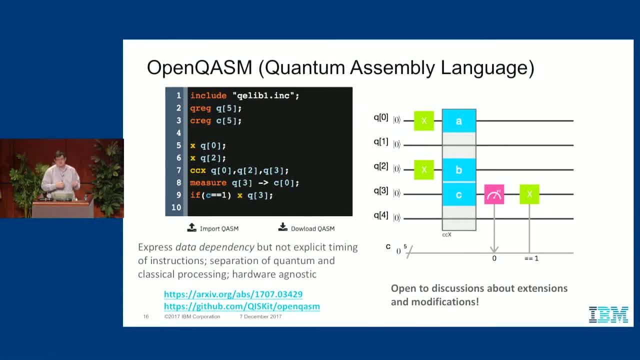 the future. this is sort of the way we'd like to think and we'd like the language to be agnostic about the hardware that's on the back end. so just a general circuit description language. We are open to discussion extension. This is open chasm, so you know, please let. 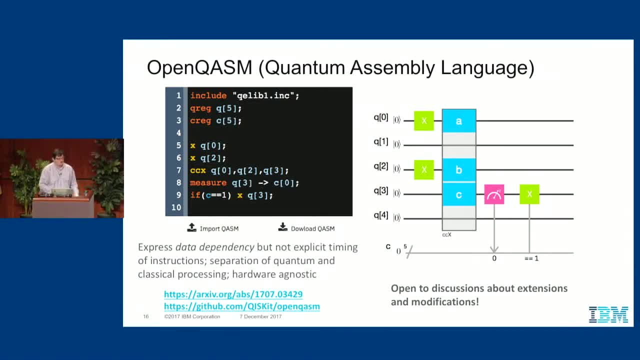 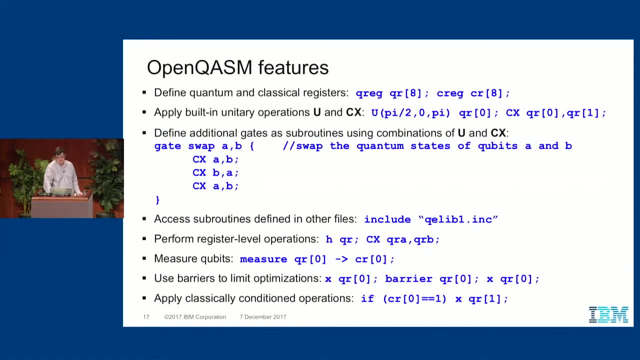 us know. if there's something you don't like, you want to change, We can talk about it. The specifications are all online, All right, and maybe yeah, I'll just say I'll just highlight a few more things. right, This is how you make gates hierarchically from other. 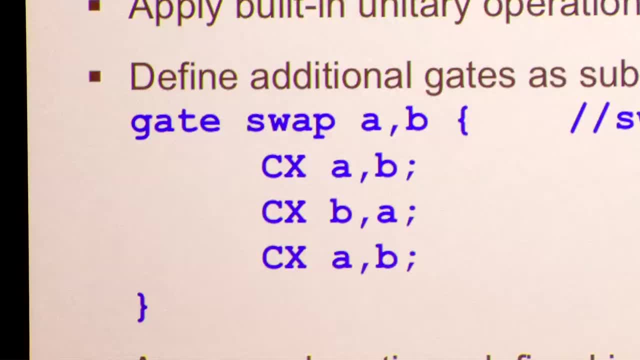 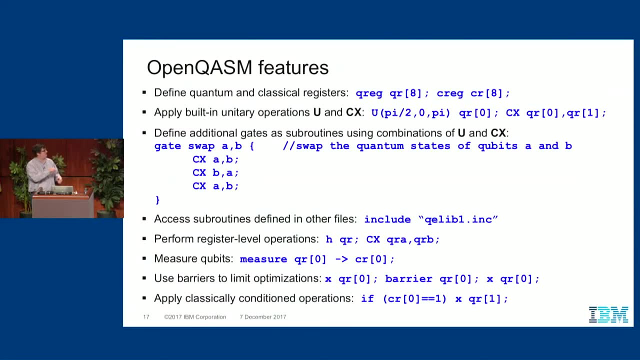 gates that you've already defined. There are some syntactic things, like you know. in some algorithms it's quite natural to apply a Hadamard in parallel to many gates, so there's a way to do that. This applies it to every qubit in this register, and there's this, so this 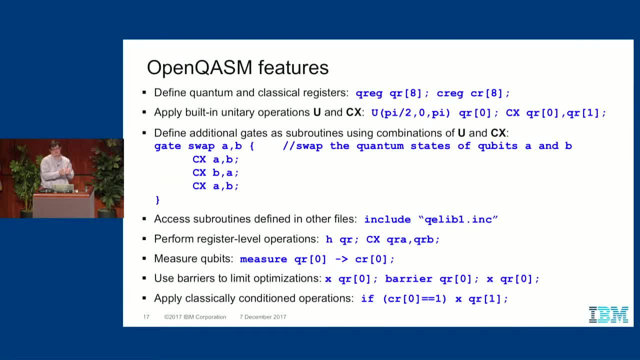 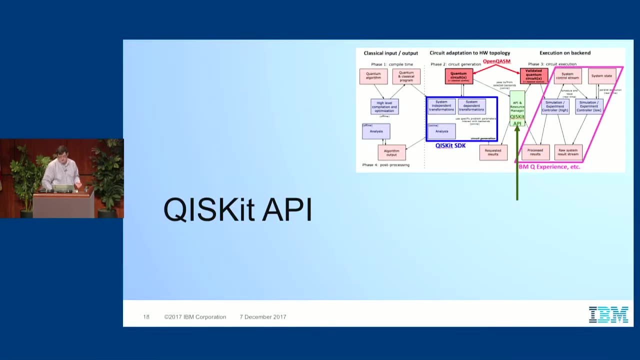 barrier instruction says you know. it says don't cross this line, right? So if I have an optimizer that's walking through this circuit, what it's going to do is it's not going to combine these two x's into identity, right? It also affects timing, All right. so that's chasm. and now? 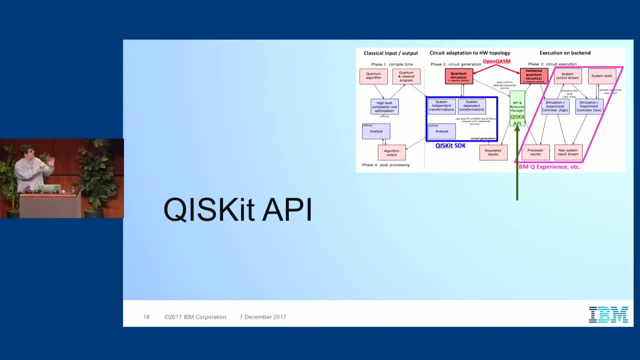 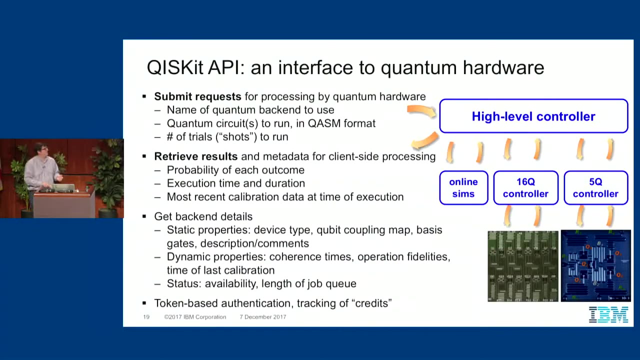 I'd like to start moving to quizkit. I'll start first with the API itself, so I'm also going to focus mainly on the Python implementations of these components. So I'll talk about the API and then I'll talk about the SDK. All right, all right, so. 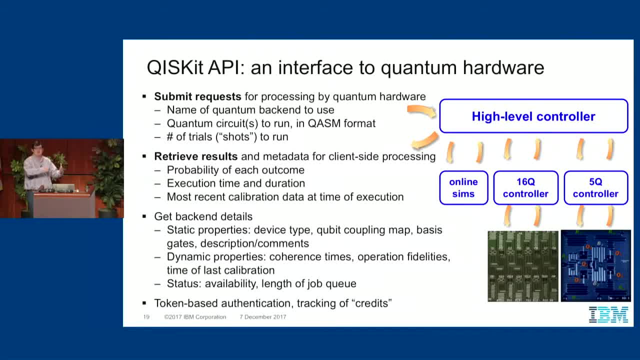 the idea. the idea is that so there's there's a web API, it's a, it's a REST API and you submit requests to it, like the backend. I want to use the set of circuits, I want to run These right. 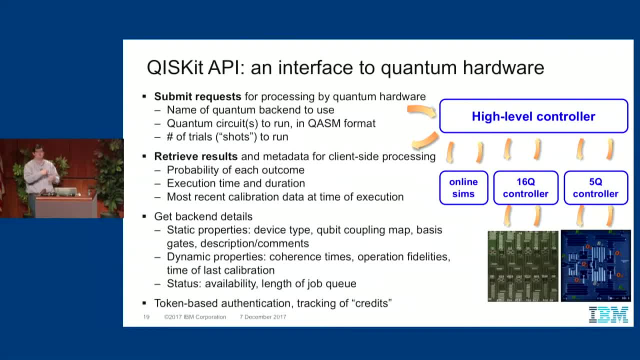 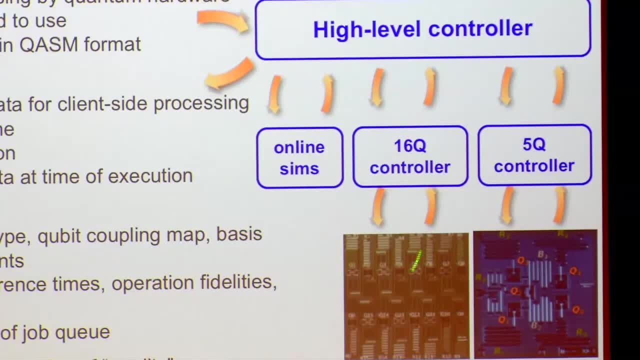 now are given as chasm circuits, and how many times to run each of them. It's pretty simple. So you submit this request, right? This, it's processed, sent to the appropriate backend device. it gets processed further, right. The experiment runs. it comes back. 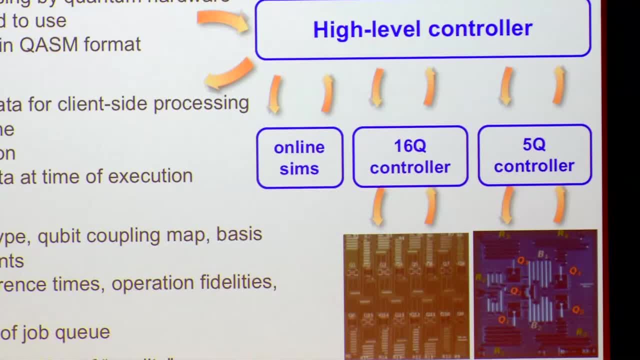 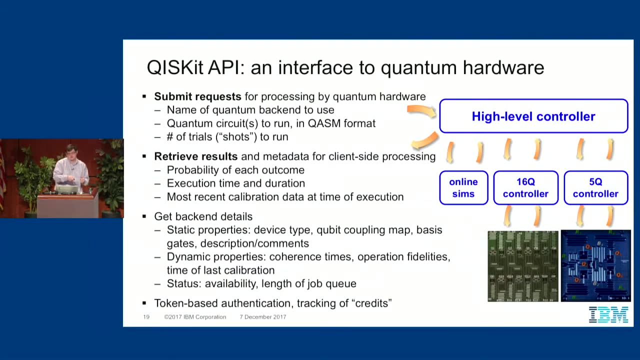 there's queuing- there are other things here that I'm not going to talk about- And after some time the result comes back to you and you can request it. And you know it includes the, the probability that you see each outcome string how long it took. other other kinds of information, What's one? 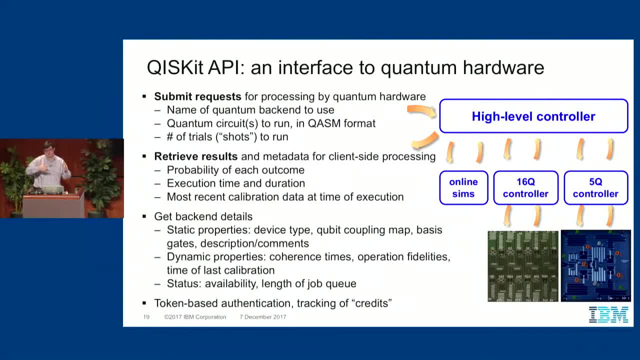 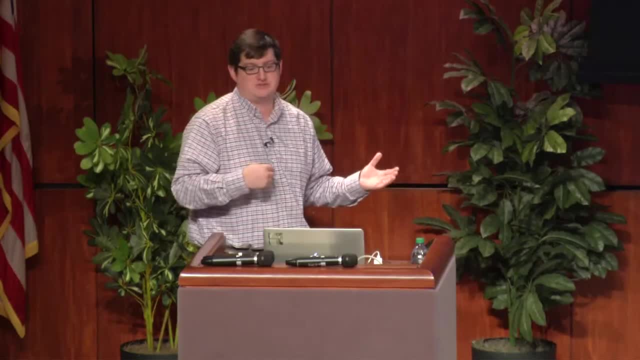 of the important pieces, though, is that it gives you a, you know, a collection of data that corresponds to the calibration, The most recent calibration before your experiment, which is always it's good to have and be able to combine with your results. You can also make requests. like you know, you can ask for a lot. 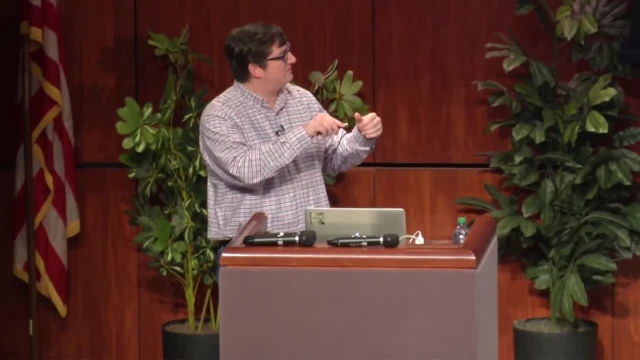 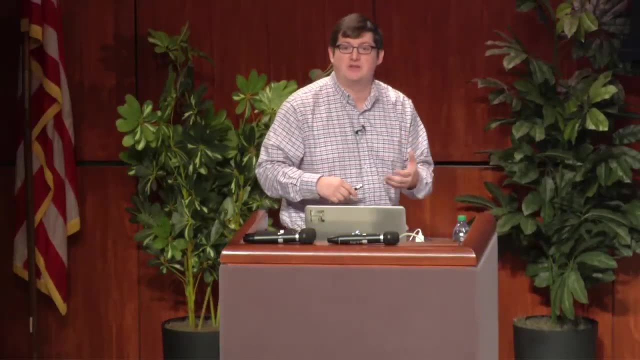 of information about each backend and some information about the queue. This is all authenticated, based on tokens. You go to the Quantum Experience website, you ask for a token and then you use the token to access this. I'll give an example in just a little bit. Okay so. 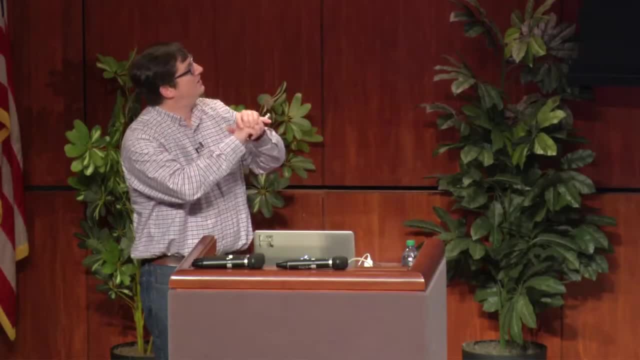 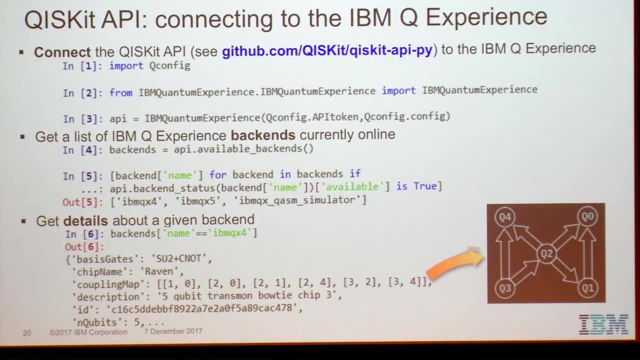 so now, now, some code, Right. so this is what it looks like. if you just want to use the API, All right. so so, bare bare minimum, I want to run something on the device. I don't want, I want to. I want to talk right to the API. So in Python, you can import this module that has the methods in it, construct an API object. you give it the token, you give it the configuration. So this, this is the URL of the Quantum Experience. I'll show it to you, to you later, And this is some you know long string of of characters. 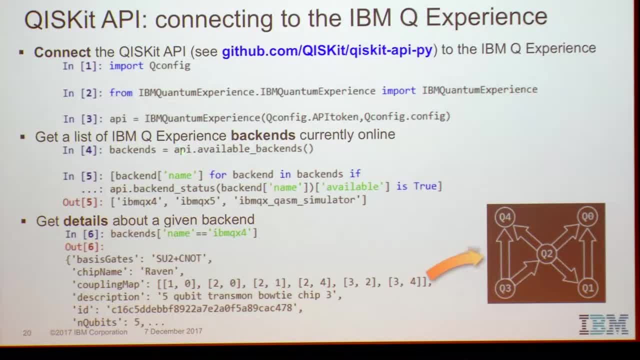 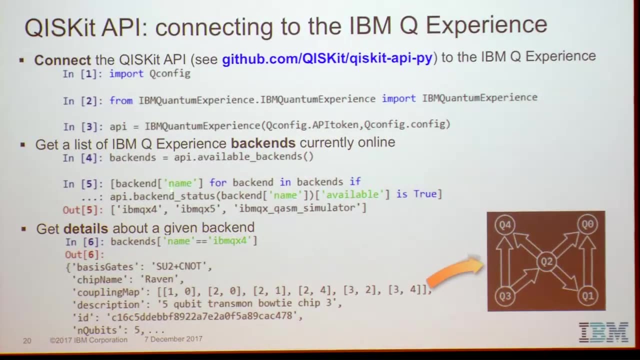 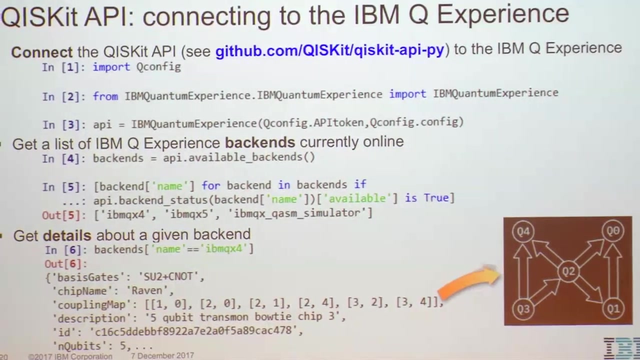 Once you've created this API, you can say what backends are, are there, And it's going to send back a a dictionary of backends And you can look at the, the names of these, So you know for each backend, let's look, look at its name as long as the backend is available, So it backends may become unavailable if they're being calibrated or if they're taken down for some other reason, right, So you can check that And this comes back and it tells us that you know. 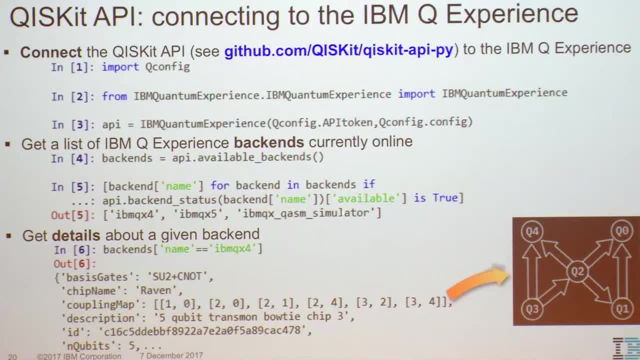 two devices are available. This is this is 5 and 16. And there's an online simulator. Okay, And if we want details, we can go into this backend dictionary and look up, look up 1. And we get all the information that's available for that backend. You know just, I mean, for example, one of the more important pieces of information is how the qubits are connected. Okay, So this says pairs of qubits on which you can do a two qubit gate, All right. 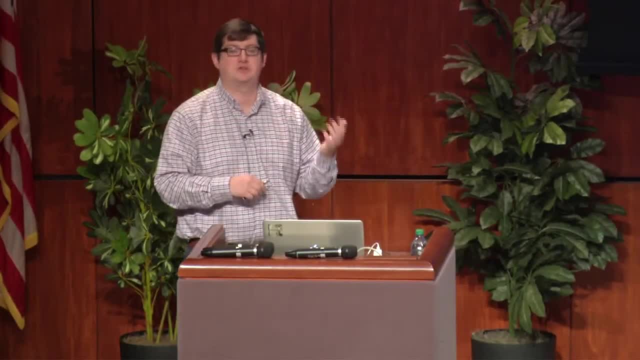 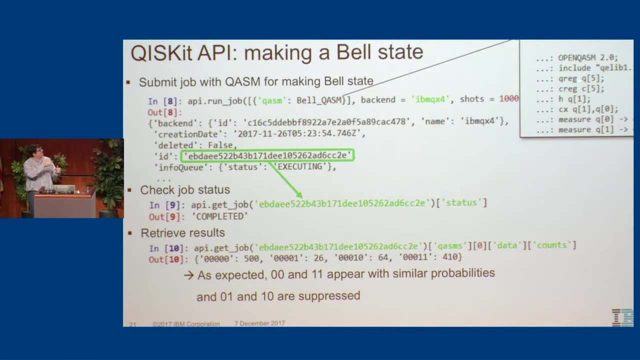 So now, if you, if you, if you want to directly use the API to run a circuit, here's how you would do it: You need to generate the chasm code. So here it is. This is code that makes a bell state right. I have two 5 qubit registers. 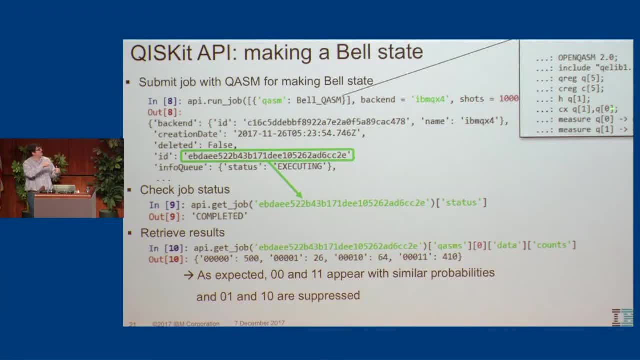 I apply Hadamard to one of the qubits, a controlled knot between that qubit and another one, And then I measure them both. Okay, Specify the backend, how many times to run this experiment, and then it goes And you get back a blob of data. 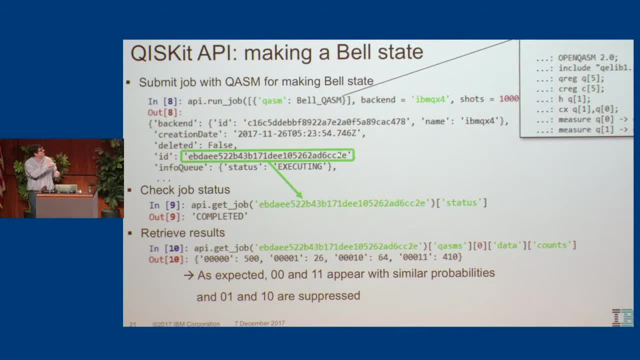 and I mean this has a lot of information in it. but what's important to follow up now is the ID of this job, So you can grab this, put it in this call and check whether or not it's done yet. 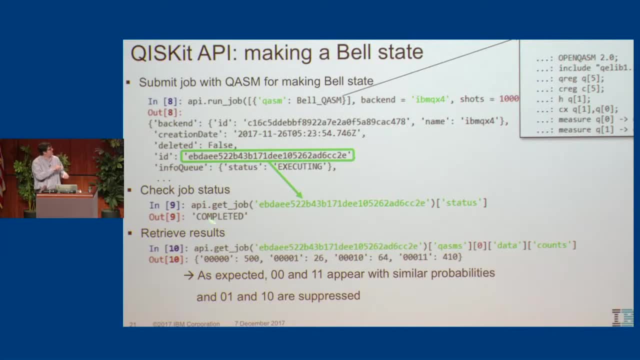 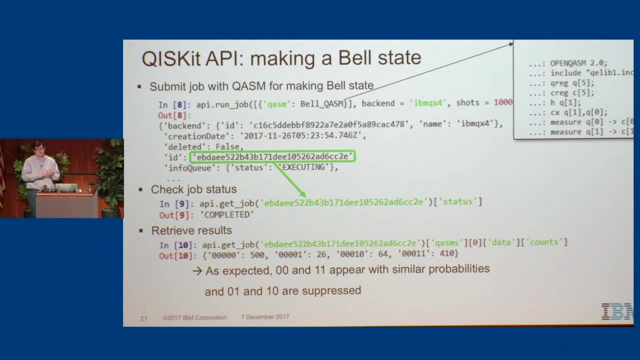 Okay, So that's it, And then, when this is complete, you can, you can go and retrieve this and this. this will contain all the information. It'll contain what was run. you know when it was run. 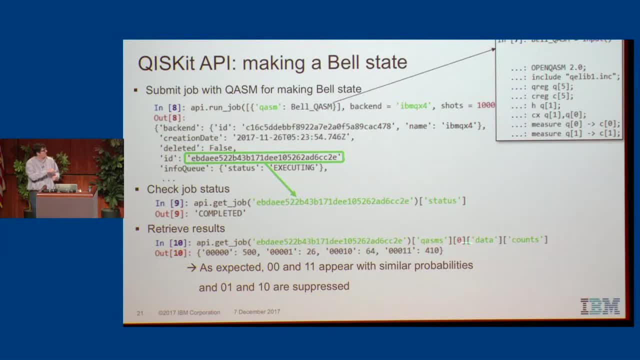 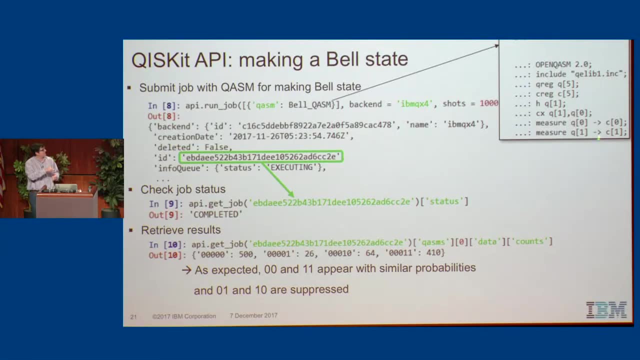 calibration data, everything. And among all that data, one of the things you can ask for are these counts. So, for each, each time through this circuit, we get a string, an output string. so the value of this register: C. 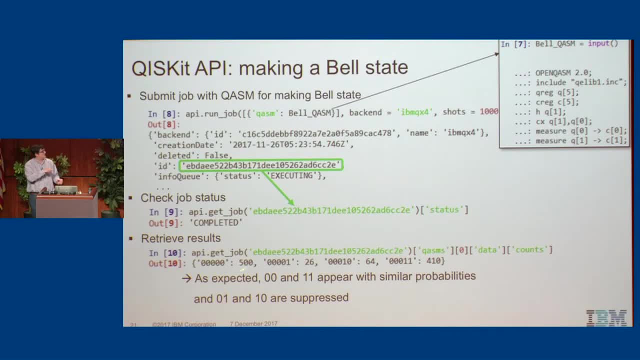 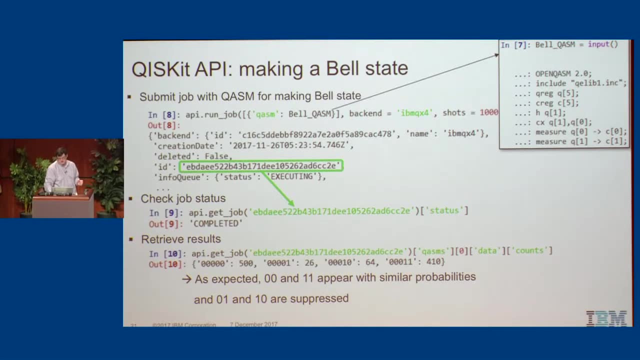 And so this is returning the value of that register C and how many times we saw it out of the total number of shots we requested. Alright Now. so so that's great. So you can run quantum circuits, you can run them through the API. 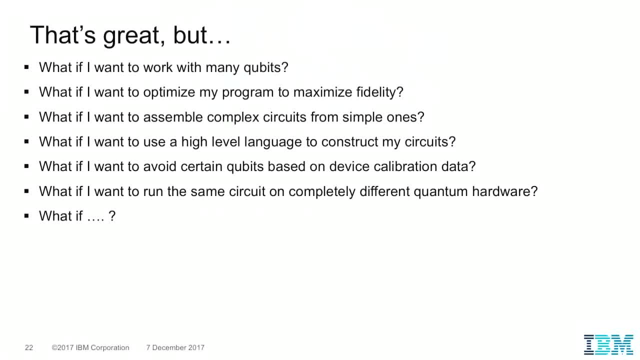 Maybe you don't want to work with the API at this level. You know what if you want to do something that's more complicated? What if you want to optimize your circuit- your circuits- first, and send them in? What if you? you know what if you want to use a higher level language? 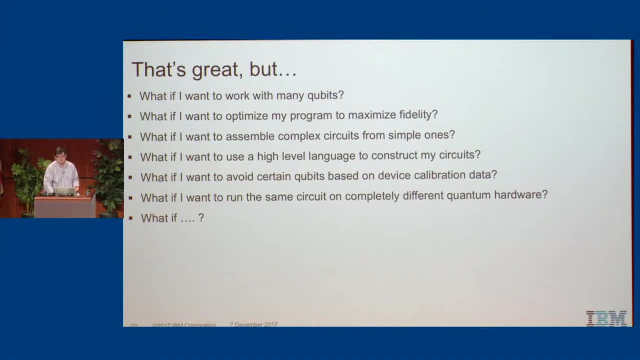 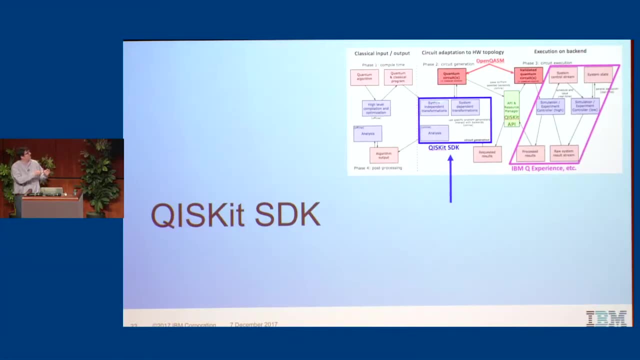 to construct your circuits. I mean, it's not very easy to to program to this API. So you know, we'd like to build on top of this, And so that's what we're doing here. We'd like to. 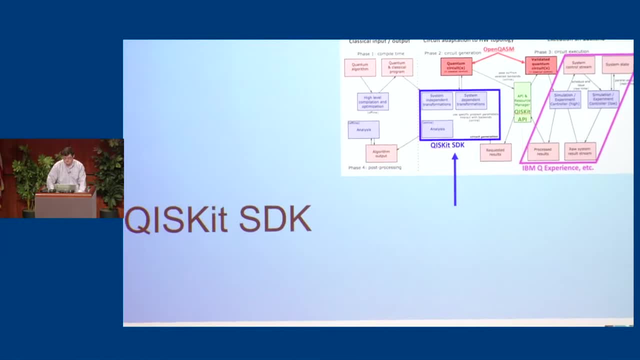 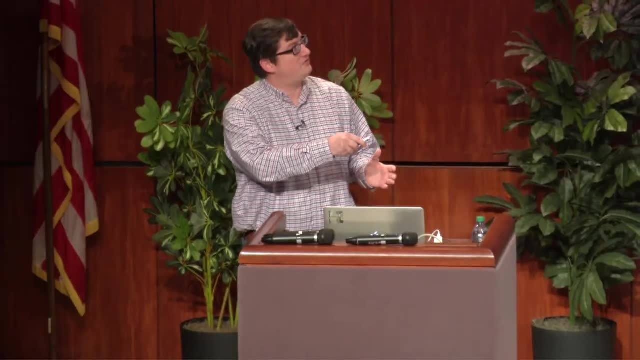 yeah, I'll, I'll just continue here, So let me go into some of the details. Alright, if you're interested in downloading this and trying any of this for yourself, everything's available, starting from here. So if you go here, 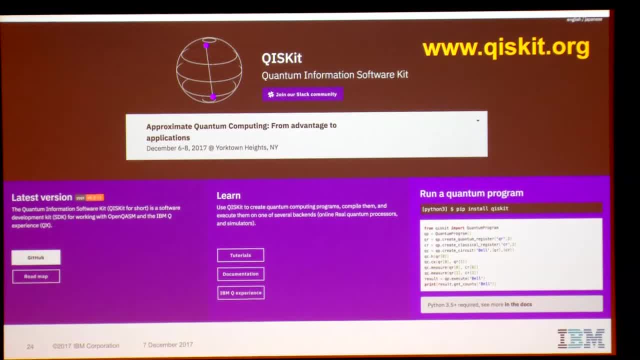 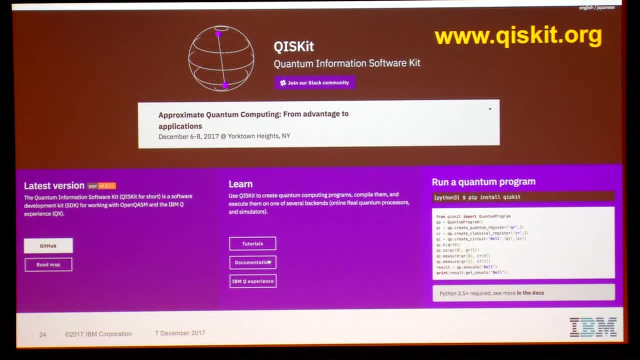 you can follow from these links to to any any of the information you need. So just to point out right, the code is all open source. It's on GitHub. There are tutorials, documentation and a link to the quantum experience directly from here. 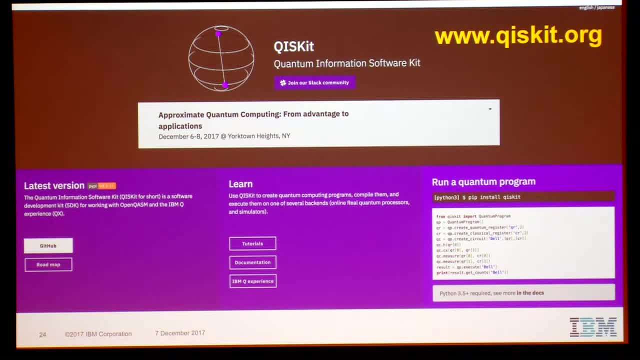 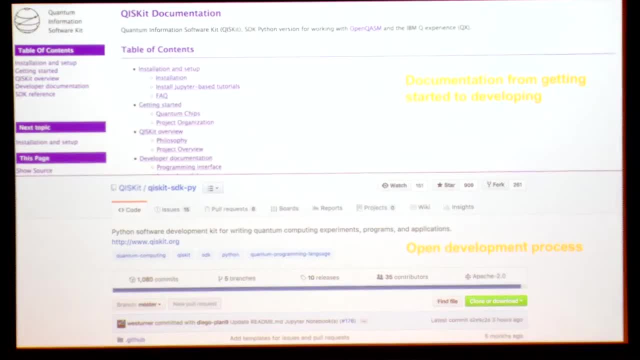 as well as how to get started. Now I'll I'll go through this in more detail in just a couple minutes. Let me highlight a few of the a few of the places you can go from this landing page. So there is documentation for this software. 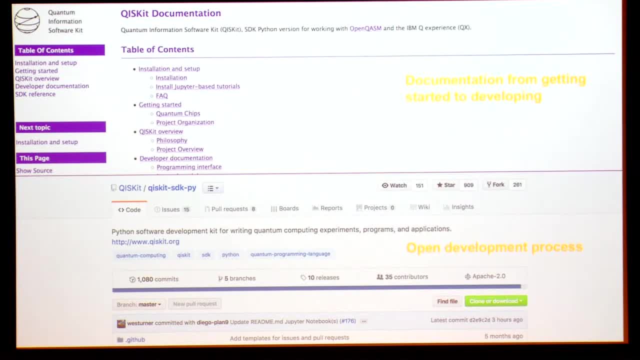 It includes how to get started using it, as well as documentation of this, of the code itself. So, whatever level you're interested in looking at this code, you can do it through the documentation And you know we've included some of our thinking. 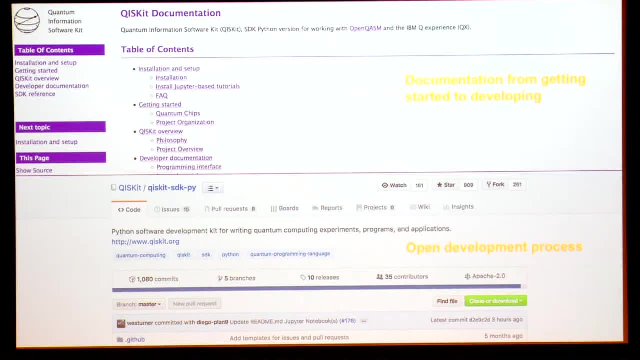 in terms of how we have currently organized the code. The, the software, is developed openly. It's all on GitHub. You can see our- our process, You can see who's contributing to this And you know the things that are currently being worked on. 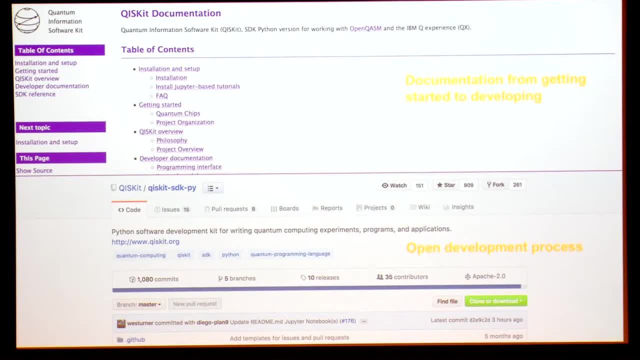 through pull requests. We've been very fortunate that people in- you know, people outside of IBM have been interested in contributing as well. You know the the flow is essentially: if you, if you want new features, you would open an issue and we would discuss it. 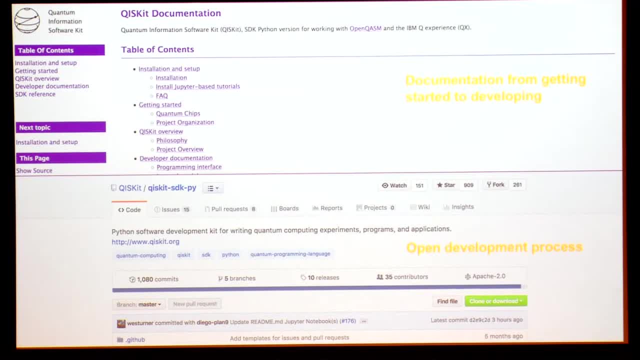 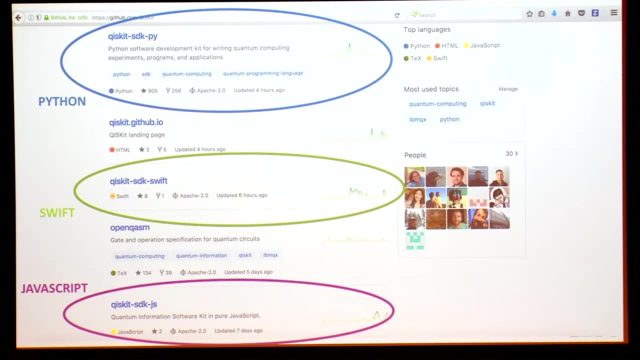 You can submit your code on your own fork through pull requests. This is your relatively standard way of of doing this. You can see some of the the files in the project for more details about how to contribute. Now I focused, and I will continue to focus, mainly on the Python. 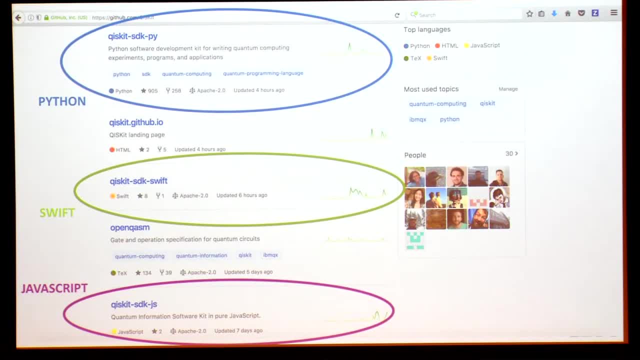 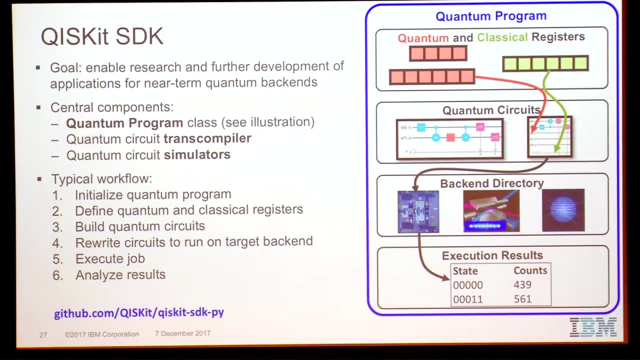 but in this project you can also see, we have a Swift implementation of this code and a JavaScript implementation as well. So if you're interested in using other languages, you can All right. All right, So the, the SDK is. 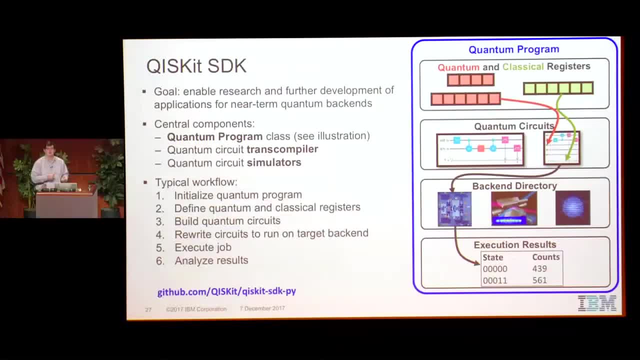 the. the quiz kit is organized around quantum program object, And this program object is a collection of quantum circuits that are all somehow related. So the way in which they're related is that the quantum program has a set of quantum and classical registers. 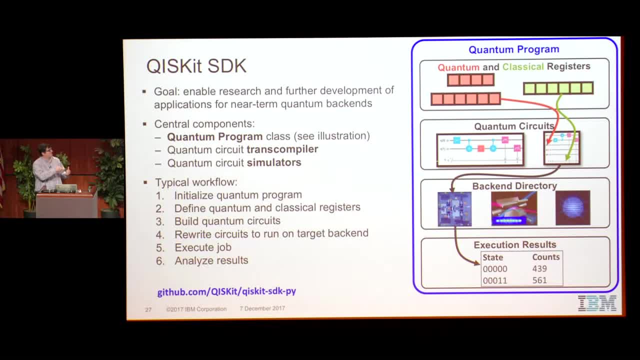 associated with it. You create those and then you build circuits and then you can run those on some backend, get the results and bring them back. Okay, In the process you may rewrite them to run on some target backend, if you. 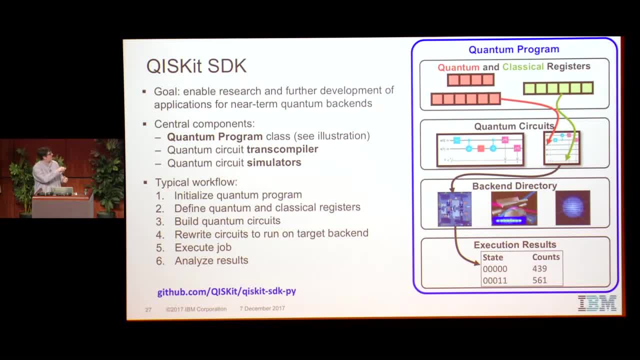 if you have a limited connectivity, All right To do that. there is a component that that that rewrites the circuits. We've taken to calling this a a transcompiler, and this is the reason we do this- is that 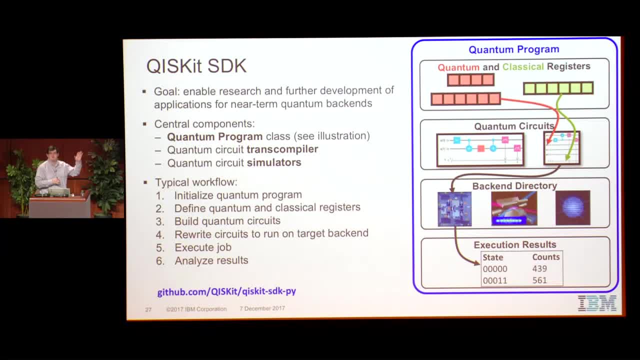 we want to emphasize that our our goal is not to go from a high level language all all the way down to the lowest level code that can run on our system. We, we want to rewrite chasm to chasm, So 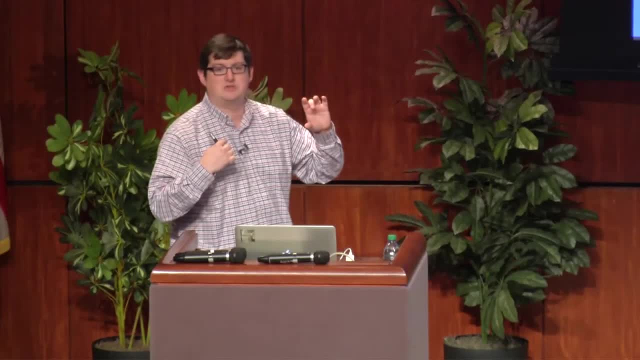 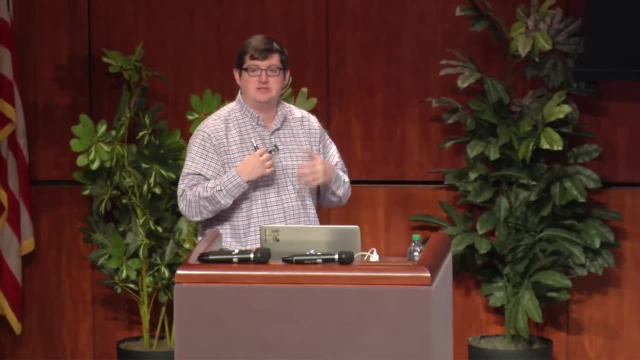 we're sort of going horizontally. It's a limited, limited scope right now. We want to take our input circuits and we want to make sure they run on the backend and we want to make sure we eliminate as many gates as possible. 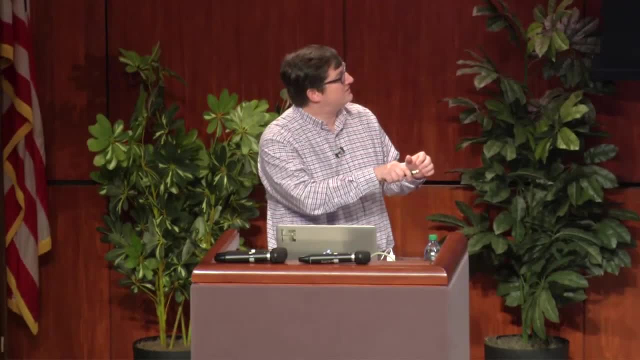 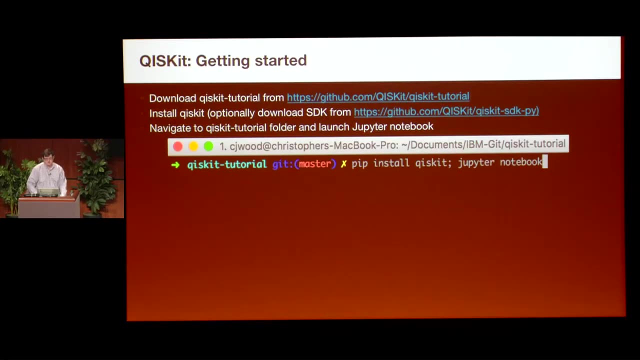 before we do that, Okay, Among the backends it includes simulators as well. So this is, the simulators we have are also part of this project, All right, So so how do you get started? All right, 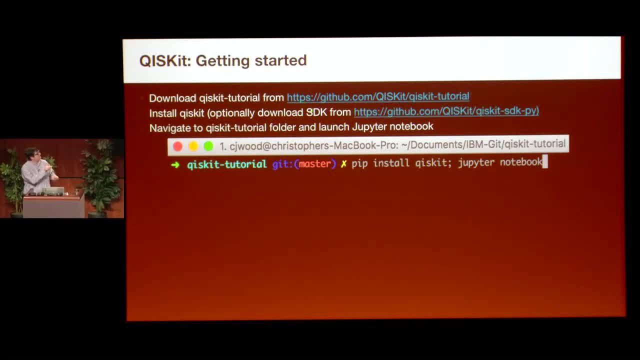 So you can. you can get two, two components, from the repository. One is a set of tutorial Jupyter notebooks, So you can grab these directly from GitHub and download them, And then there are two ways that you can download the. 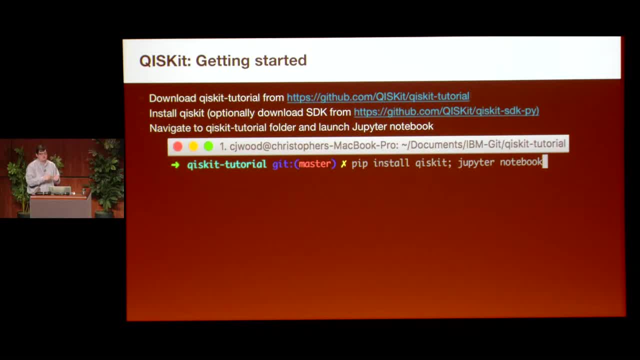 the this quiz kit software. If you're interested in in writing code or looking at the code, you can. you can grab it from GitHub Or you can simply run pip install and you'll get the latest stable version of it. 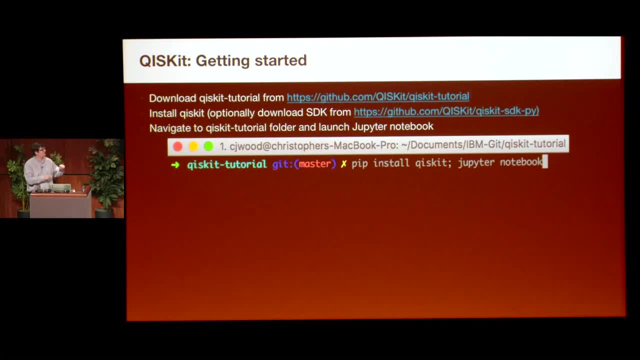 Okay. So then if you want to get started, if you have, say, Anaconda installed and Jupyter installed, then you just install quiz kit and then start Jupyter. And if you want to use an online device, so if you want to use one of the quantum experience devices, 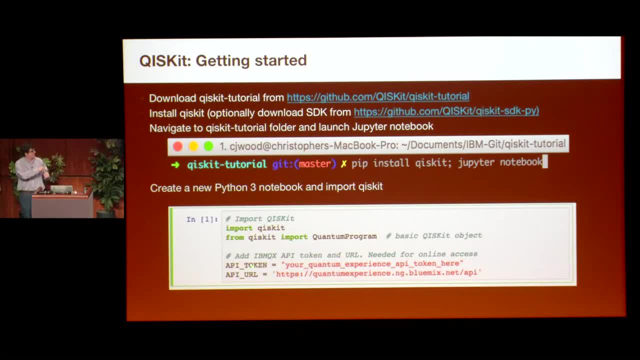 there's one other step you have to do. You need to go to the quantum experience website under your account and get the API token there and then substitute it here, So you'd put in your token and put in the quantum experience URL. 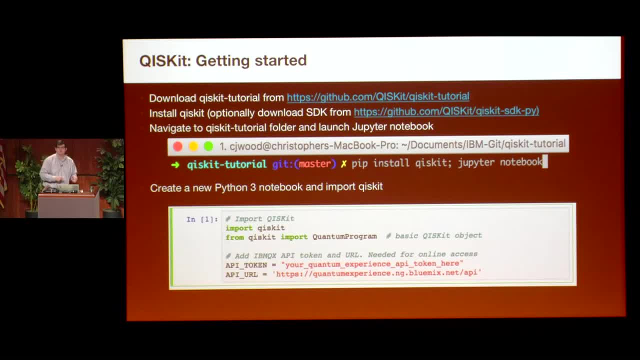 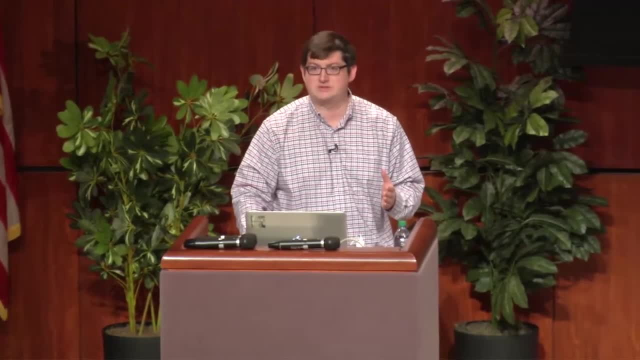 Okay, These are also in a file called qconfig in the in the repository. You can fill them in there if you like to. All right, So now I'll walk through in the last, in the last part of the talk, a very simple example from start to finish. 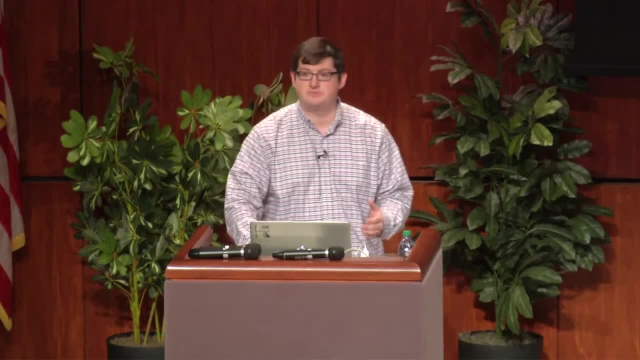 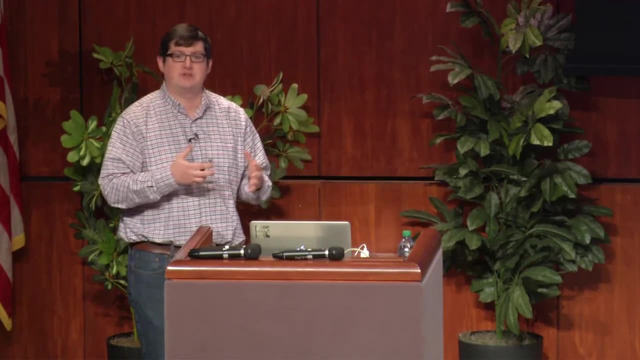 and a couple ways of of looking at what comes out of that example. All right, All right, So the first thing we need to do is make this quantum program object that will encapsulate everything we're doing in this experiment. All right, 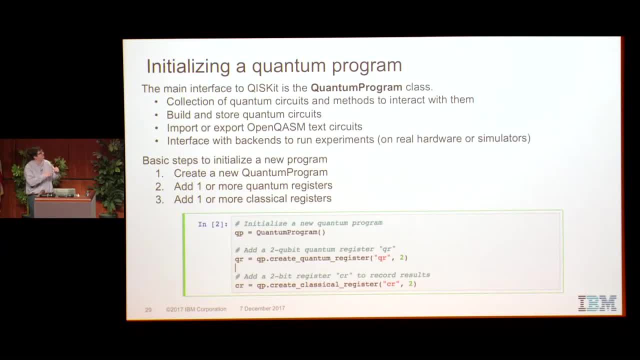 And this has methods that are generally you know they're, they're in the category of, you know, constructing these circuits and manipulating them. It lets you import and export to this chasm text format And you can interface with back ends. 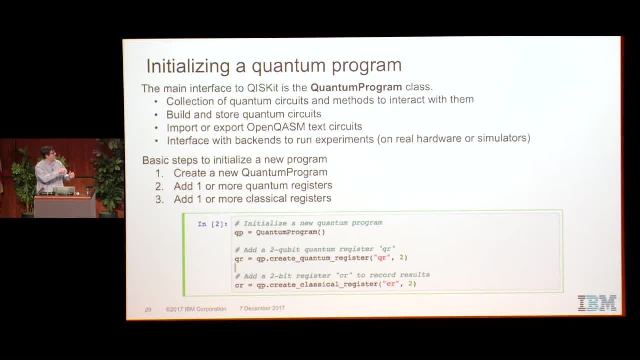 obviously, Anyway. so this is what it looks like to get started. You make this program, you create a, a quantum register, or two or three. This is the name that will appear in the chasm text and this is the Python object to manipulate it. 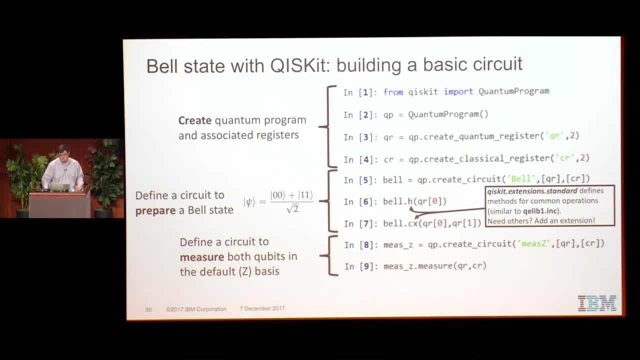 similarly with the classical registers. All right, So then this is what it looks like: to create a, build a basic circuit for a bell state. So make a program, create two, a two qubit register and create a classical register for the results. 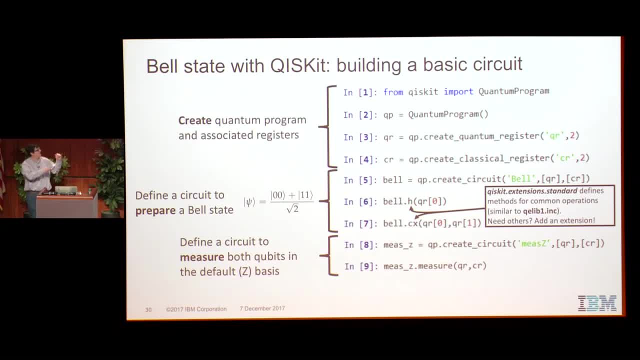 Okay, So now we have all the objects we need. Now we can create a circuit bell that we'll use to build up, build up the circuit right, And on this object we can apply gates that so these gates live here. 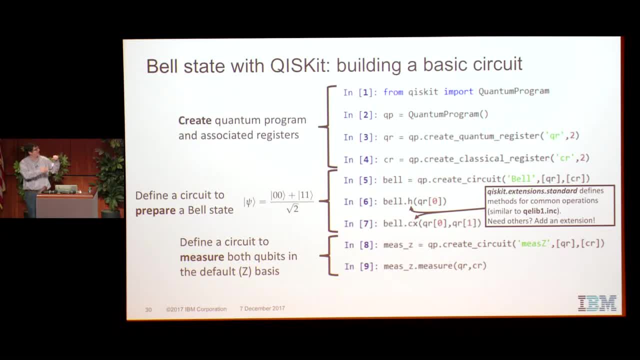 They live in something that we call the extensions And you can, if something's not there, you can- add new extensions and they add new methods onto these circuit objects. All right, I'll say more about it in a second. All right. 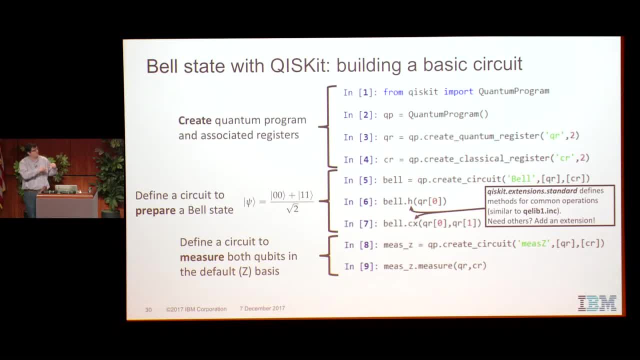 But this had a margin, so let's go back to make this state. Now we'd also like to measure it, and we may want to measure it in several different ways, So let's begin by measuring it in the Z basis. 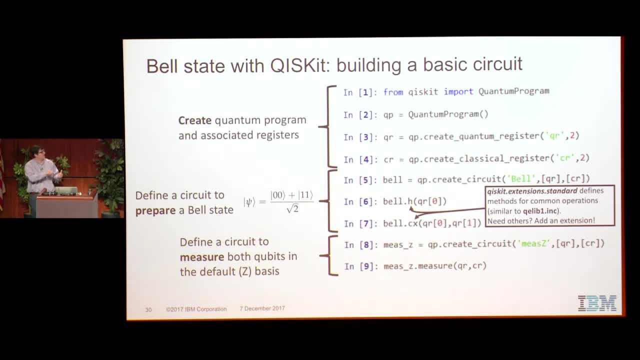 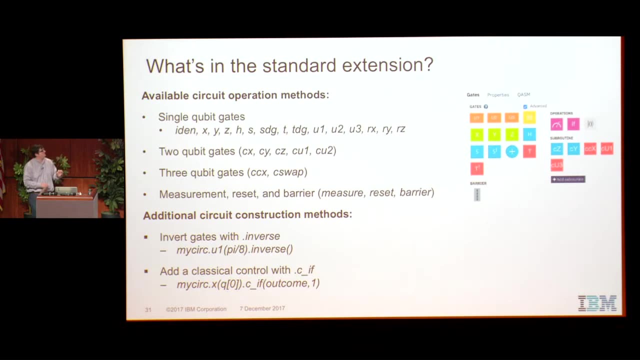 So we'll make another circuit. It uses the same quantum registers And here we just measure all of Q into all of C. All right, All right. So let me just say a couple words about what's in this standard extension. The short answer is that: 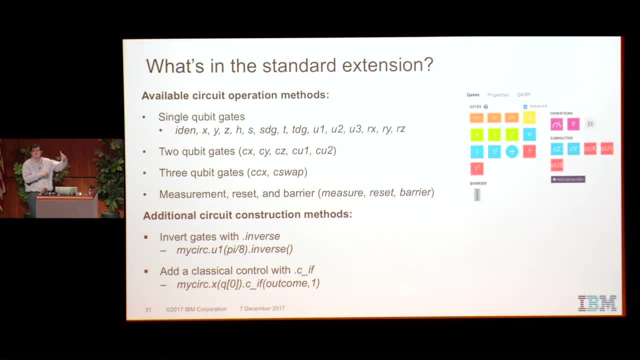 everything that is in the you know advanced on the quantum experience. all the gates that are there are in this extension. It's more or less what you would find in a quantum computing textbook. So you know the single qubit gates that you're familiar with. 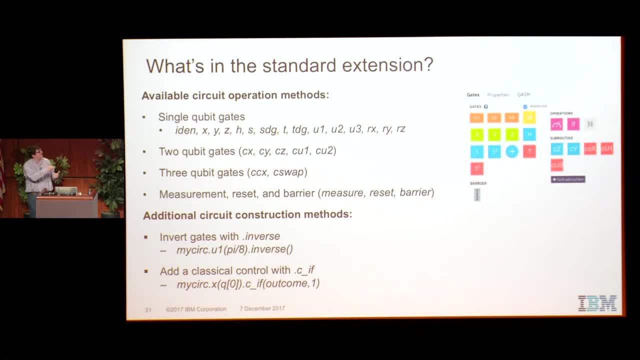 like Clifford plus T. These are the U gates that are fundamental in our system right now. Two qubit gates: These are controlled versions of these single qubit gates. Toffoli measure reset. Reset is not supported on the hardware right now. 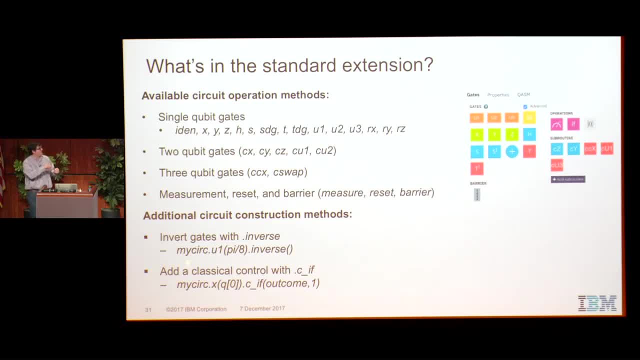 Okay, And then there are a few other construction methods and this will grow. Right now it's relatively basic, but you can take a gate, apply it and then invert it, And you can add classical controls to the gates. This will work in the simulator. 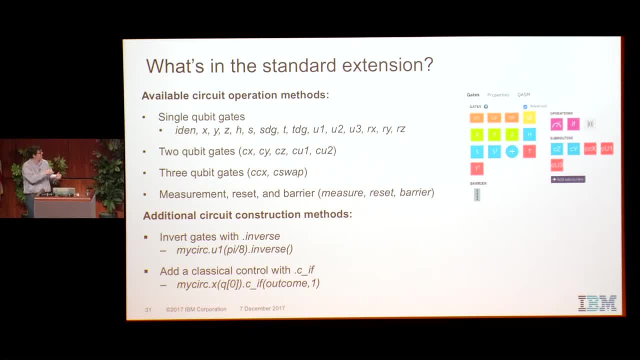 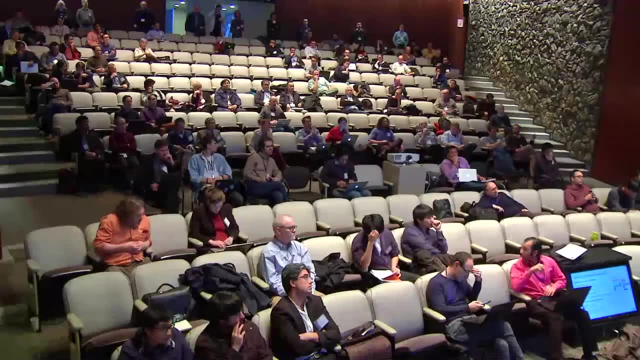 but again, not on the, not on the experiment. Okay, So that gives you some idea of what's there. Excuse me, Sure, Does a three qubit gate actually work on the back end like that, or do you have only on the simulator? 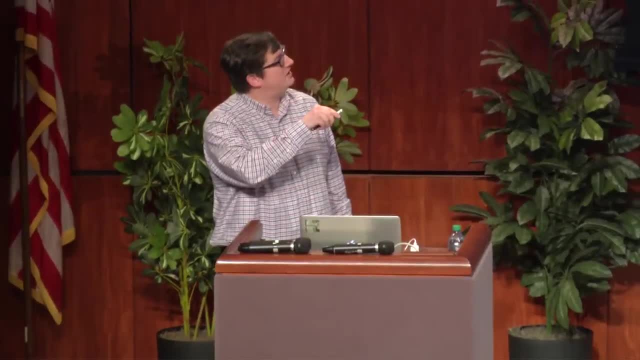 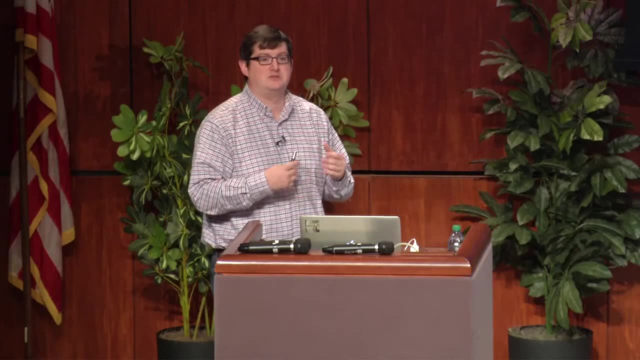 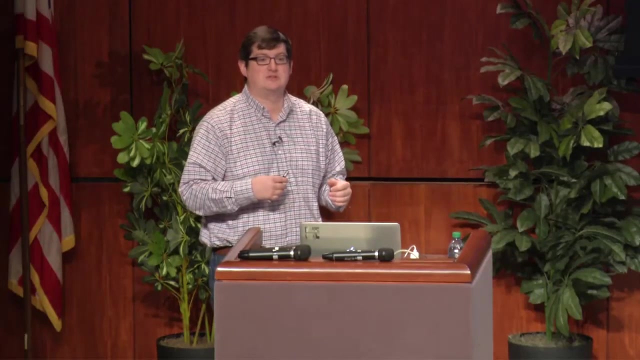 The, I believe the three qubit gate. the three qubit gate should work through the through the through quiz gate. So, because it will be, I'm sorry On the actual hardware, Yeah, I believe it should. So it should be mapped down to two qubit gates and single qubit gates. 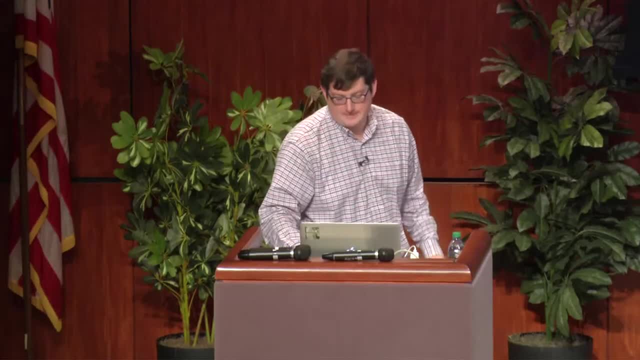 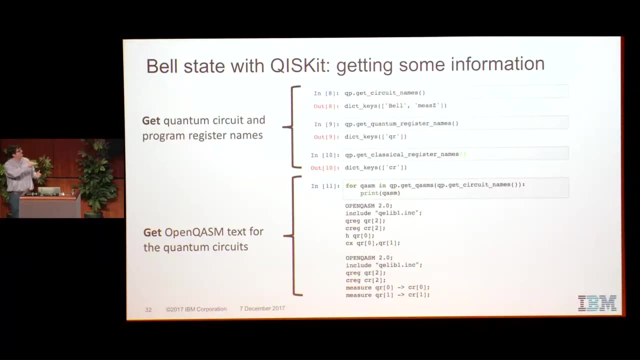 and then those should be mapped onto the hardware. Yeah, All right, So we've constructed these circuits. How do you get some more information? There are some methods to access this right So you can say: what circuits do I have in this program? 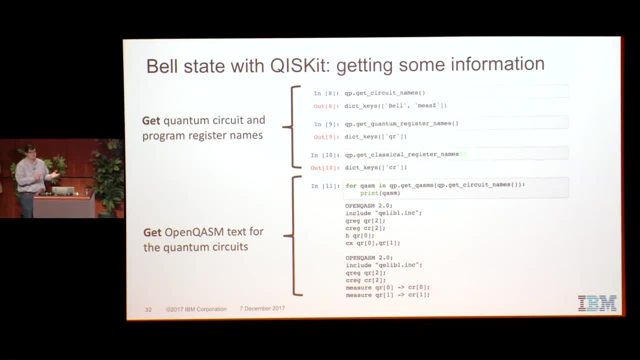 What registers do I have? What classical bits do I have, Things you might need to know, And, if you want, you can ask for those circuits back in chasm form and they come back in essentially the same way that you programmed them. 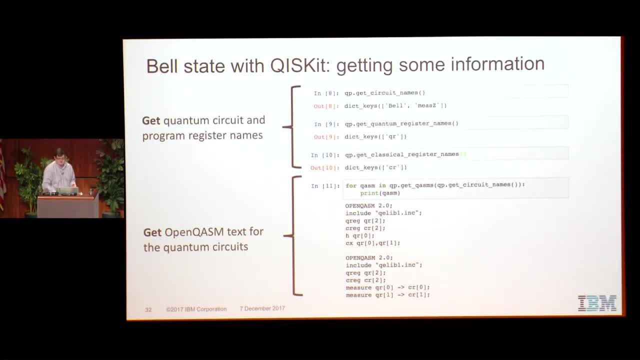 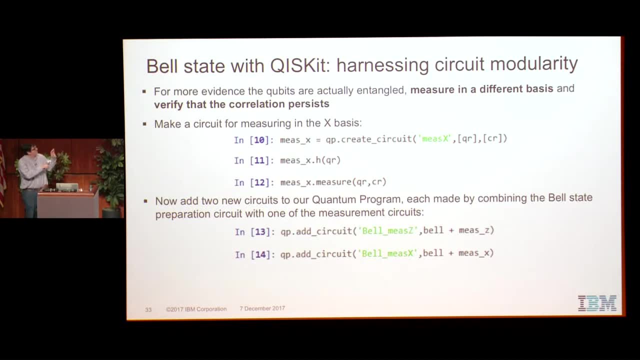 You know they they're not rewritten in any other basis. Okay, All right. So for this bell example, you want to measure in more than the Z basis, because you want to see that you, that these qubits really are entangled. 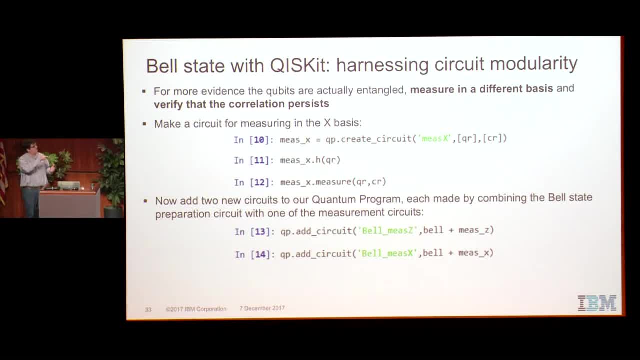 All right. So to do that we we may want to measure, say, in the X basis, So we can create a new circuit to measure X, apply Hadamard to that register and then measure it. And now we can take these: 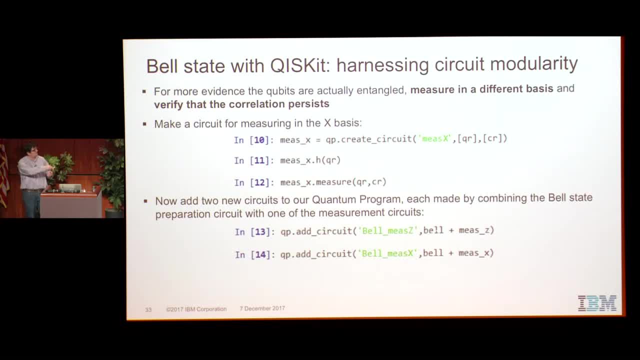 these pieces and compose them. So there's a plus operator that acts on circuits. So you can begin to stitch together more complicated circuits from these basic pieces. So now we, we build the two circuits we're actually interested in: running, make the bell state. 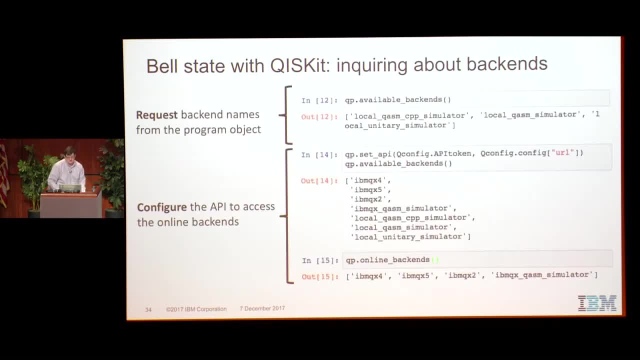 measure it in the Z basis, make the bell state measure in the X basis. Okay, Now we want to run it. So we say: well, what backends are available, If, if we, if you just type this without setting up anything. 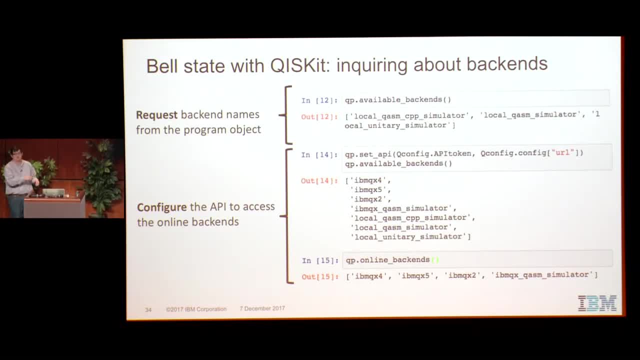 what you would get back is the list of local backends, So on. on my machine this is two: two Python simulators and a C simulator. Okay, And if you set the API and you make the same call, added to the list. 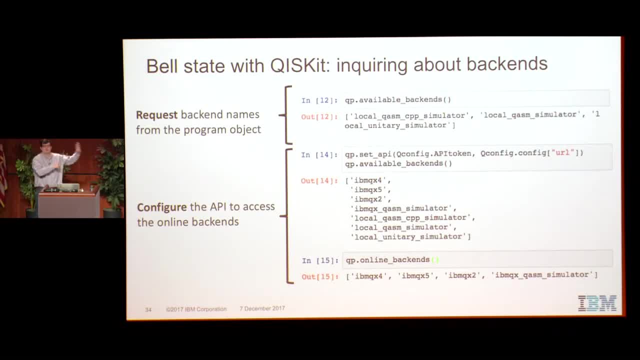 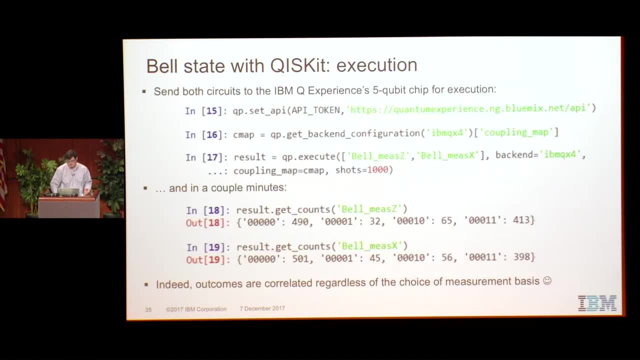 this list will be all of the online backends as well. So the simulator that runs remotely and the quantum experience devices, And of those you can ask for the ones that are, that are the online backends. Okay, So now let's run the bell. state example: 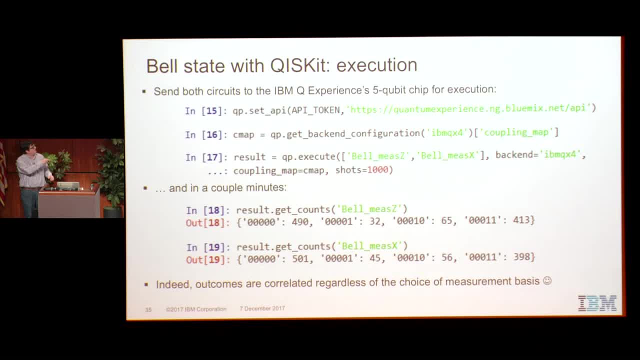 All right, We set up the API again. Now this, in this step, we're going to say is: how are the qubits connected? So give me this map of couplings. So ask for the backend configuration. get the couplings. 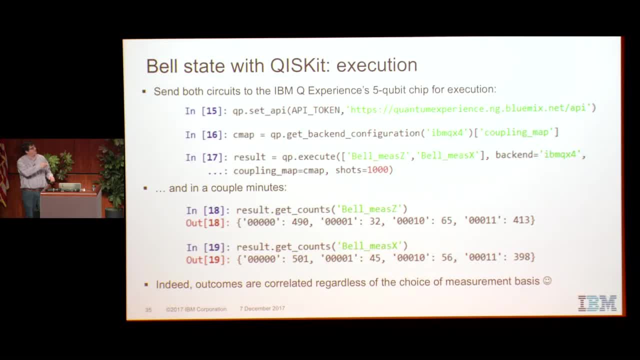 And now we say: run the Z measurement circuit and the X measurement measurement circuit in one job. you know, put them all together and send them to through the API at once. And here's how the here's how the qubits are connected on this qubit. 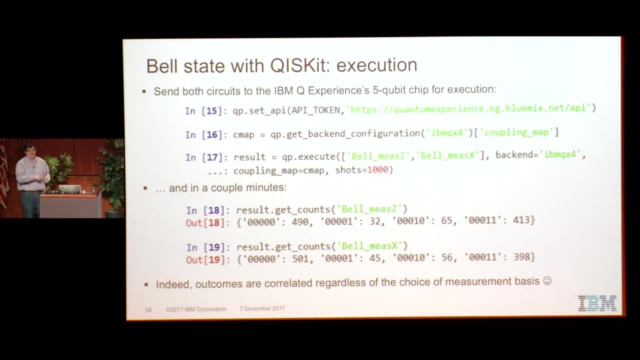 So let's say you have a two X four device, run this a thousand times for each circuit And you know this will go through the API. It'll come back. This, this calls blocking, but there are other calls that'll. 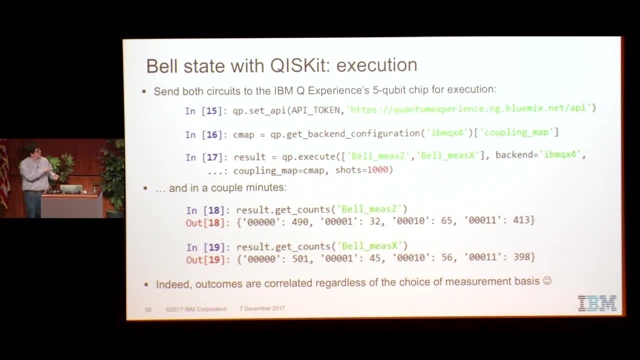 you know, submit everything and you can come back later and and check, And so after a while you can ask this result. object for the results for each circuit. So in this case, measuring in the Z basis, we see some output like this from this five qubit device. 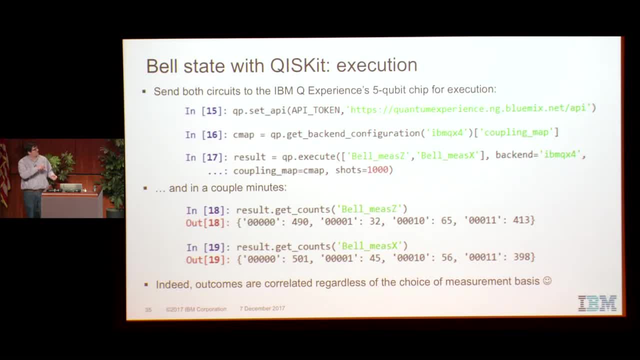 And in the X basis, we see this, And I mean what you can notice is that most of the outcomes are zero, zero and one which you'd expect for a bell state. And these in the middle, these are errors. Okay, 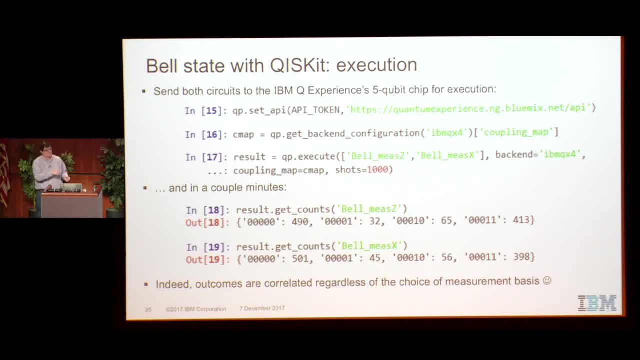 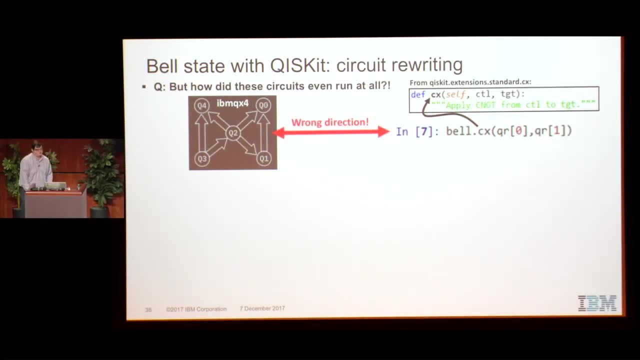 Similarly, in the X basis, you see something just like that. Okay, So you see them correlated, regardless of the basis, you measure it All right, All right, So right. I mean I alluded to this earlier, but this: 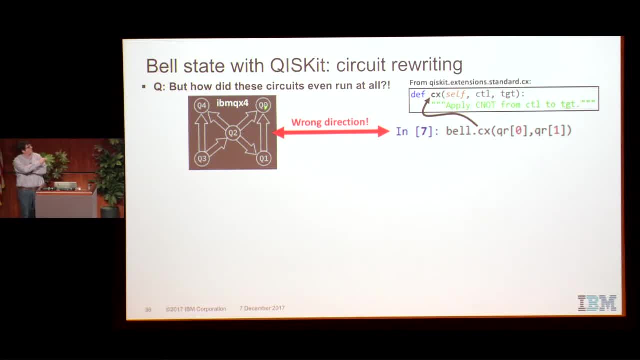 if you, this instruction we wrote down is a CNOT from zero to one right, But the hardware, this gate direction, has to be from one to zero. So I mean, what happened is that when you called execute, it called some code that rewrote the circuit for you. 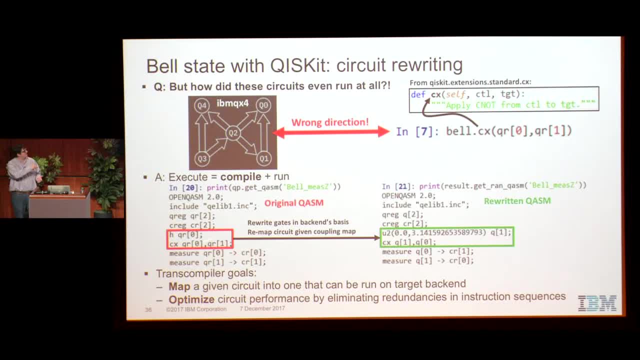 So in the original chasm there was a Hadamard and CNOT from zero to one, And now the, the one and zero labels just got flipped over here And the relabeling happened on the measurement Okay, So that's an example of 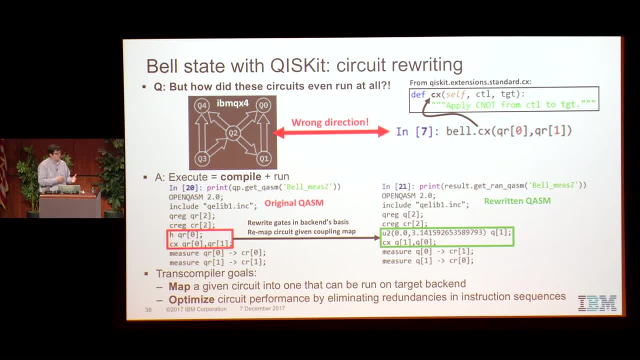 of this rewriting backend that we're working on Again. the goals for this piece are to map the circuit onto one that can run on whatever backend we have in the future or now, And also to try to eliminate instructions so that we have a more accurate 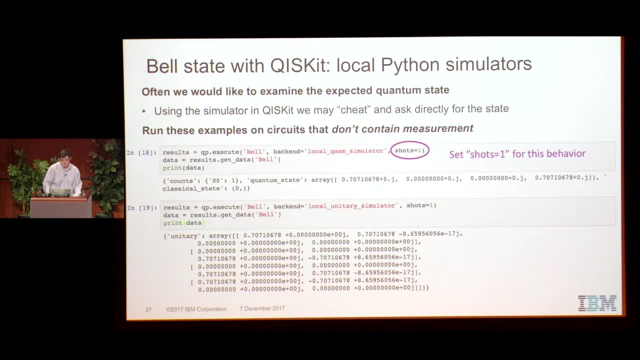 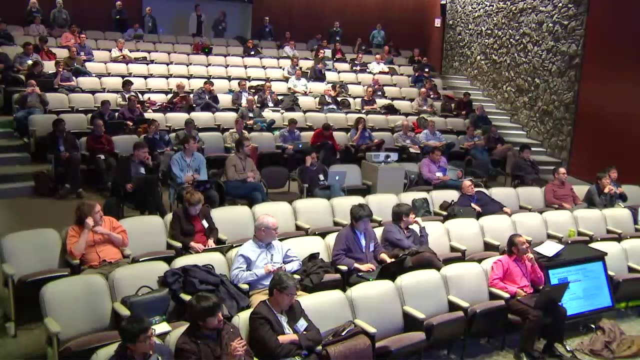 results at the end. All right, So now we can run. we can run the experiment, We can look at these histograms. Oh sorry, Go ahead. You have a question. So how much of such an embedding would you do in general? 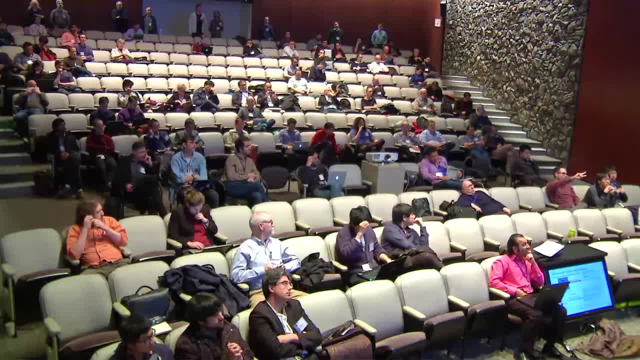 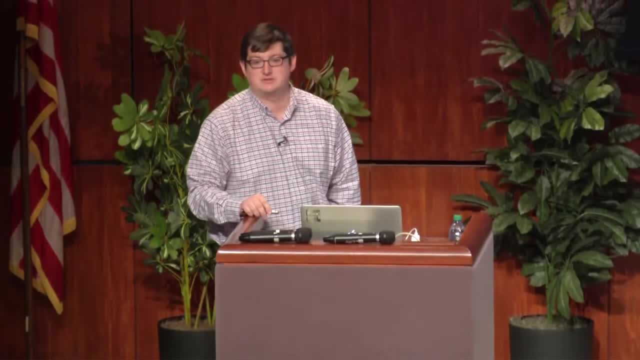 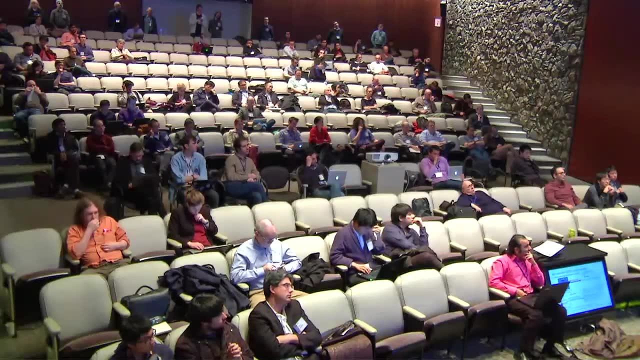 I'm sorry, By this change that you here, you only change the direction, but it could be way more complicated. Yes, It usually is more complicated. Yeah, Yeah, I'll say a few more words about what it does, but yeah, 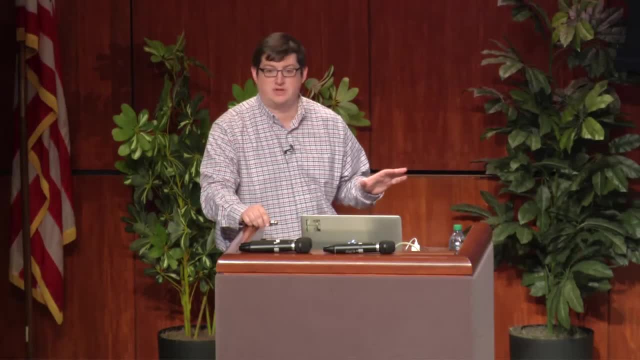 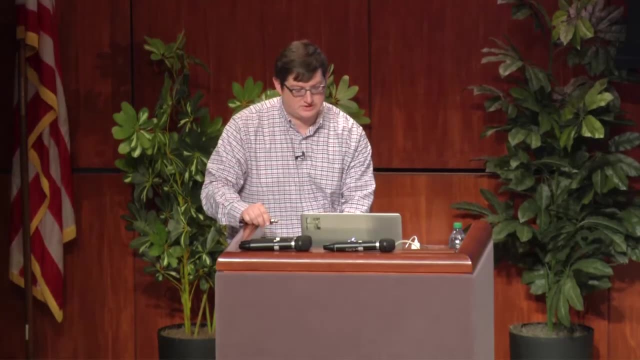 it's right now. right now, what's there is not close to optimal, but it works for any layout graph. Yeah, I'll say more about it in a second. All right, So we ran the experiment. Let's run a simulation. 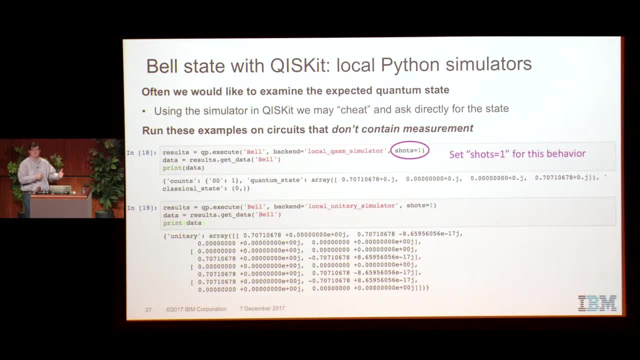 Now in the simulation, of course you ask for the state. We don't have to take shots. So if you'd like to do that, what you can do is you. you can take the same circuit. You don't have to do any of that again. 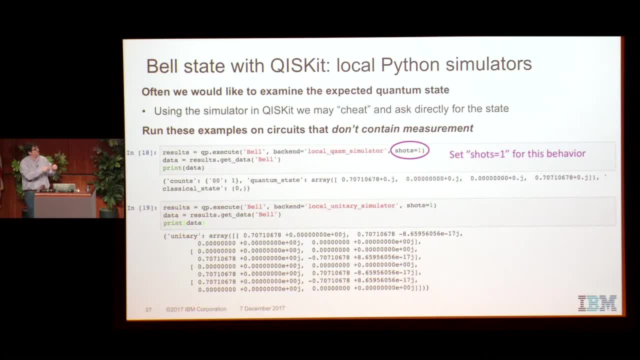 but you can just change the name of the backend And whenever shots is set to one here, it will just compute the state vector or the unitary or you know whatever the mathematical object is that you want from that simulator, And then you ask for the results. 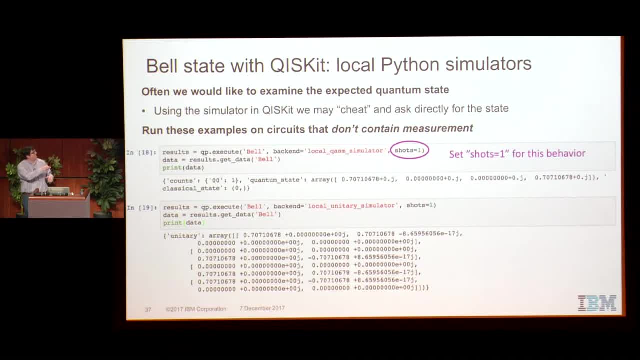 And in this data right, in this case, for this local simulator, it'll give you an array that corresponds to the quantum state right. This is zero, zero and this is one one. Okay, You can do the same thing if you want to know the unitary operation that you applied. 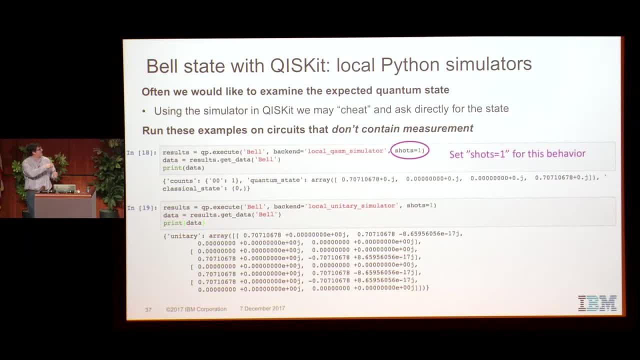 All right. So in this case, well, I mean you can, it's very easy to read. but it's there. Both of these Python simulators are you know they'll work for small circuits We have you know. 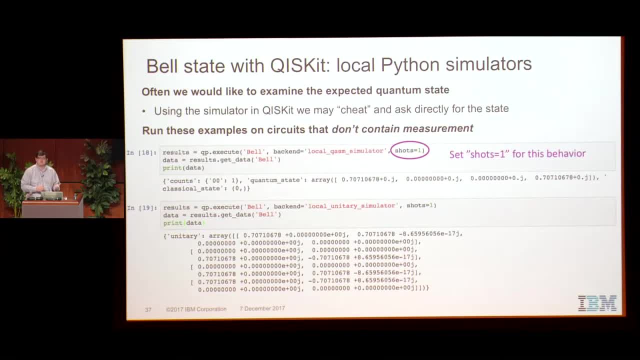 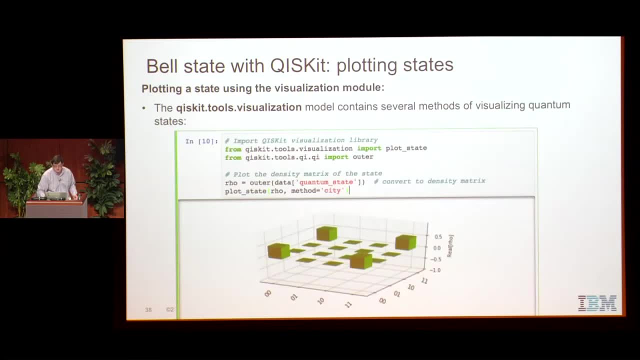 coming quite soon some C simulators, And you know we also need a very fast simulator. You can use the online simulators as well. Okay, So there are. there's a tools module in QuizKit that includes some plotting. 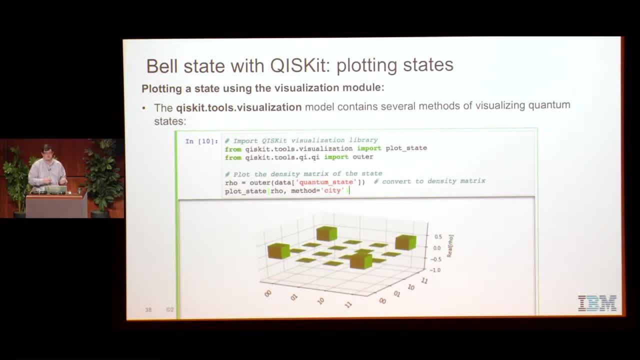 It includes some other useful functions And we'll be extending this, but let me just give an example from here. All right, You can construct the density matrix corresponding to that quantum state from the previous slide And then, and then plot it. 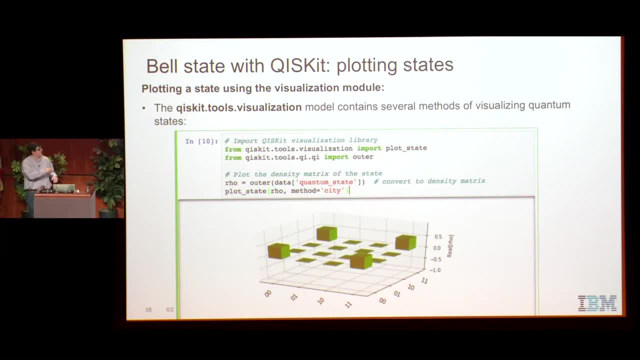 There are a couple different ways you can view it, but this is a pretty standard way to do it. This is a pretty standard way of looking at this. This is the this city plot, So you can see the the main diagonal of the density matrix. 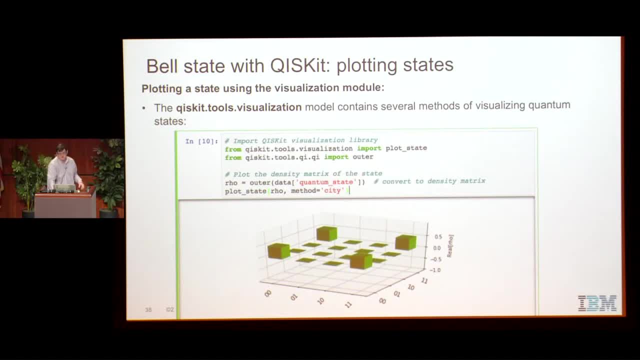 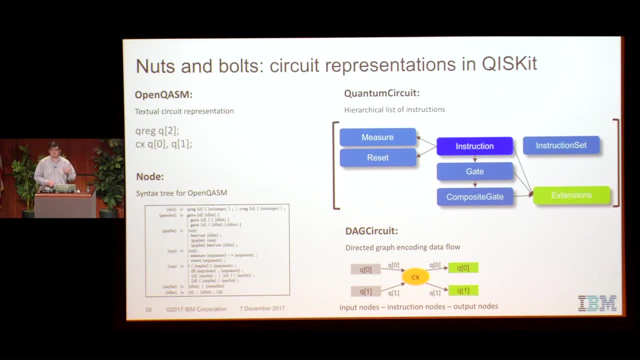 zero, zero and one, one, and then the coherences. All right, All right. So I'm going to take two slides, just in case you're curious to to know what's underneath, what's behind this, what's the structure of the code? 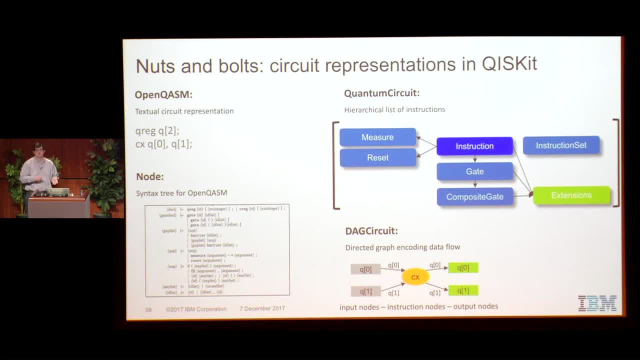 There are four representations inside QuizKit for quantum circuits and we move back and forth between them as we need to, And you know, in in the future, the well, let me, let me. I'll say what these are first. 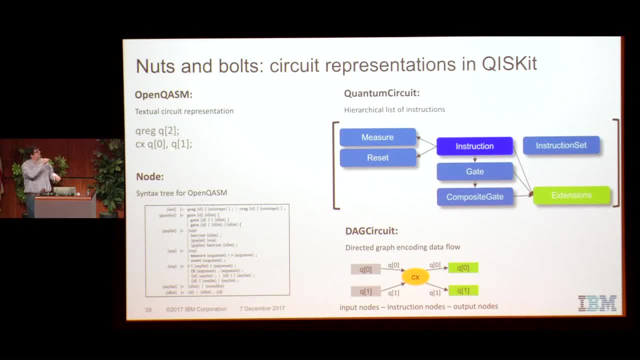 and then I'll make my comment. All right. So the main, you know, input representation is chasm text. All right, And at when this is input, it's parsed right. You get some syntax tree corresponding to the grammar of chasm. 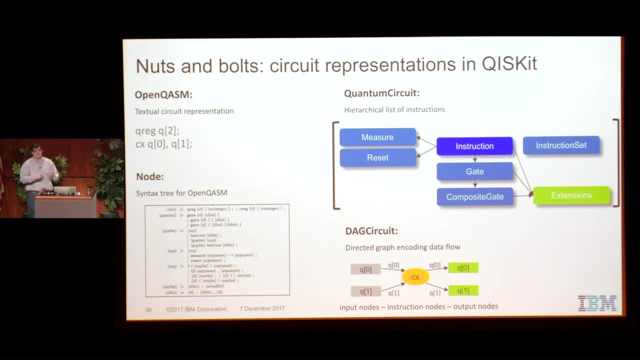 And then from here we build a quantum circuit object. And this is just a. it's a hierarchical, hierarchical list of gate objects. All right, This is, I mean, it's, not too surprising. There are instructions, there is a hierarchy of objects so that we can manipulate each of these instructions. 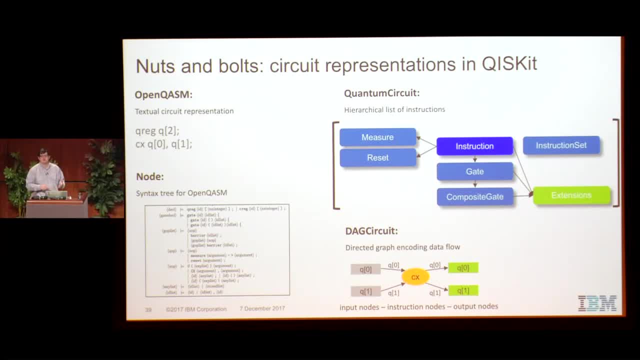 Okay, When we want to rewrite the circuit, it's very natural to take the circuit and express it as a directed graph. So something like this: you have a bunch of input qubit nodes, you have nodes for each gate and you have output nodes. 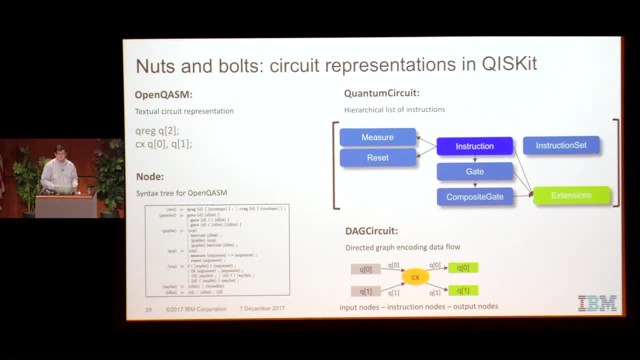 And now you can walk through this, and I mean, it's a natural way to express the circuit when you need to rewrite it. Right now, these, we move back and forth between these as we, as we please. in the future, Our focus is going to be 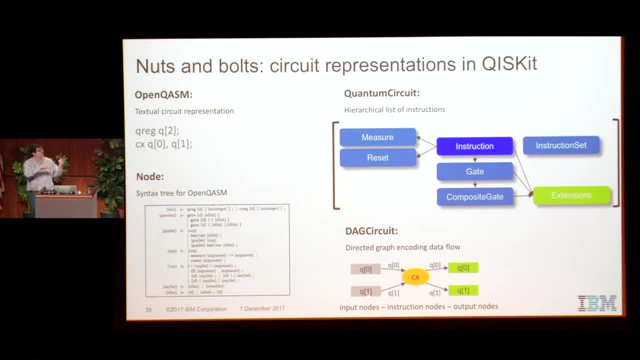 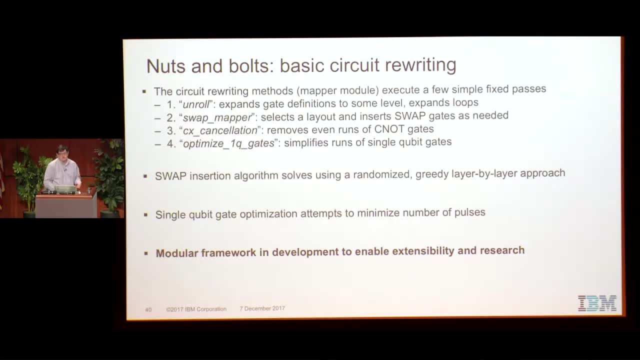 to go to this representation, stay here and move over to this representation or others that we may need as we rewrite the circuit. All right, And just to comment on you know what's underneath this, this mapping process Right now. 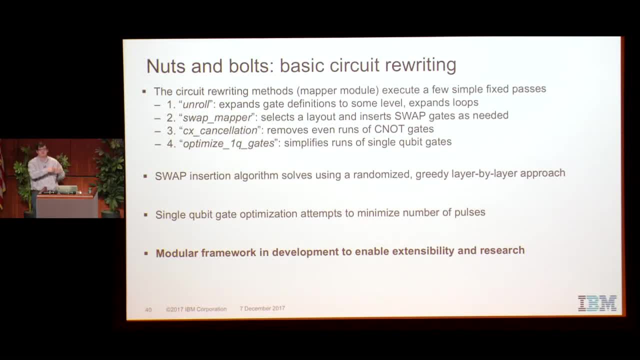 this is. this is what's here. It's a fixed, a set of fixed passes. It's just four simple passes And it, you know, it, gives you a circuit that will run on the device. This can be improved, But here is. 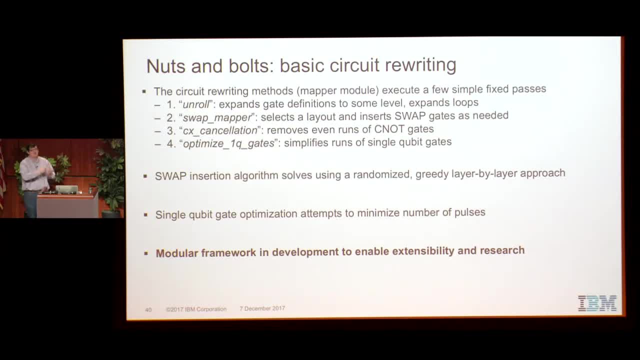 here is what is there. So we take this, we take the input chasm, we expand all these gate macros. Okay, So now there. now it's written in terms of CNOTs and these U, sub, U, sub J gates. 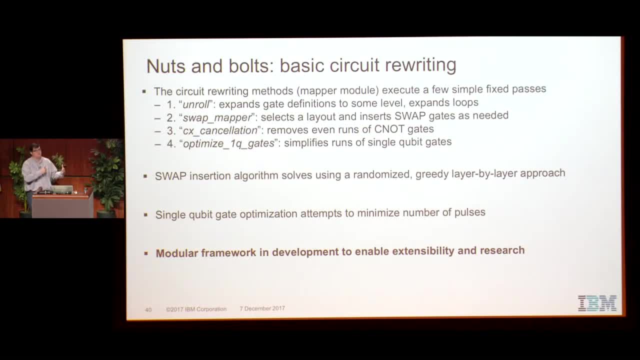 This goes to a a swap insertion algorithm. It uses a randomized greedy layer by layer algorithm to fill in swap gates to apply the permutations between these layers, And then this introduces some redundancy. So we try to clean that up a little bit. We remove runs of CNOT gates. 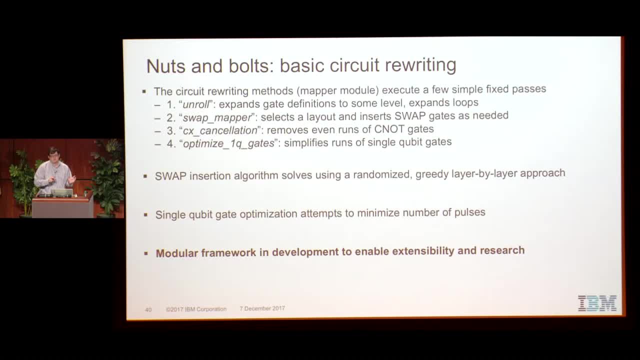 And then we optimize runs of single qubit gates that come from this. All right, And that's that's all we do, All right. This, this last method, attempts to minimize, you know, for each, for each run of single qubit gates. 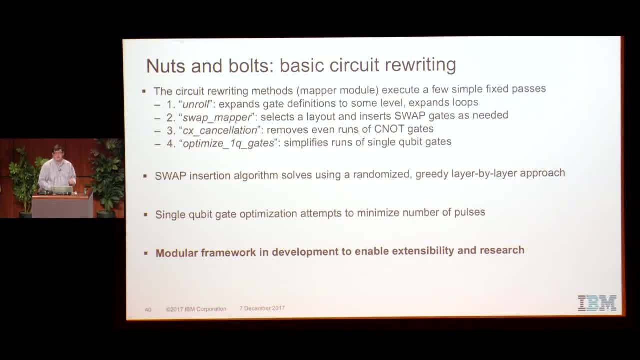 give you the minimum number of pulses to implement that gate. Okay, The way we're moving- hopefully you'll you'll see this in the coming months- is a more modular framework, something that we can build on and extend and use for our research. 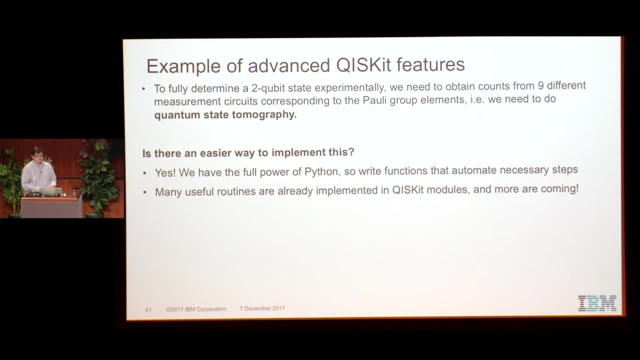 All right. So in the last couple of minutes I just want to talk about some more advanced things you could do with QuizKit, All right. So if, if we wanted to characterize the state coming out of the experiment, one way to do this is with quantum state tomography. 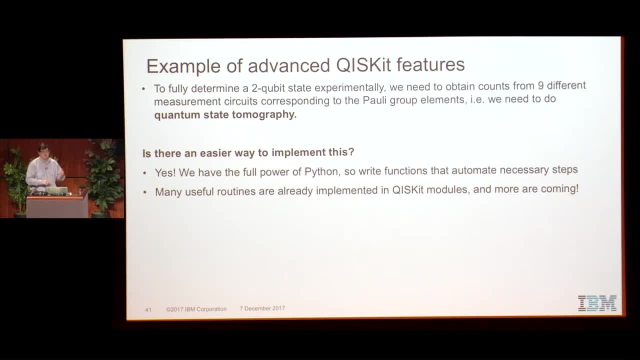 And in that case we need to make, we need to append many different measurements after building the spell state, And of course, we're doing this in the higher level language like Python, so we can just write the functions. we need to automate all of this and 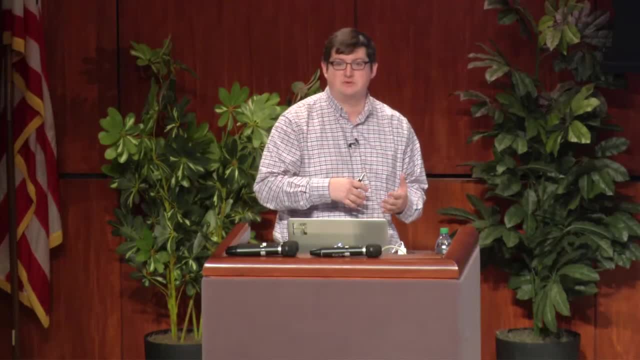 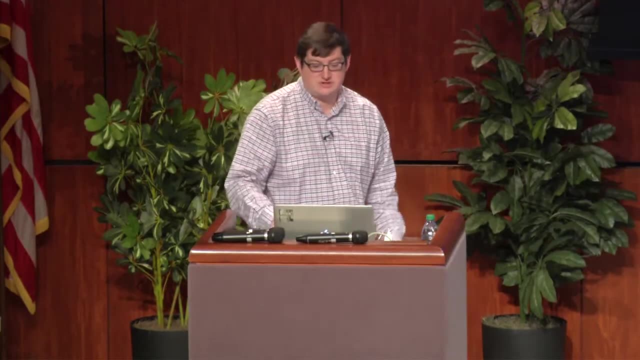 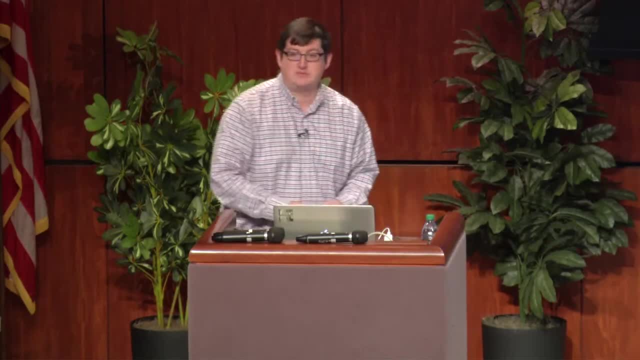 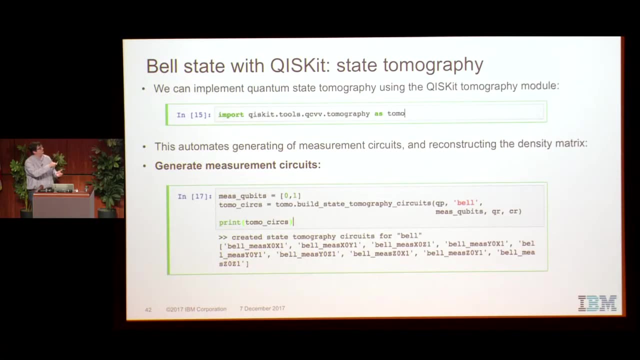 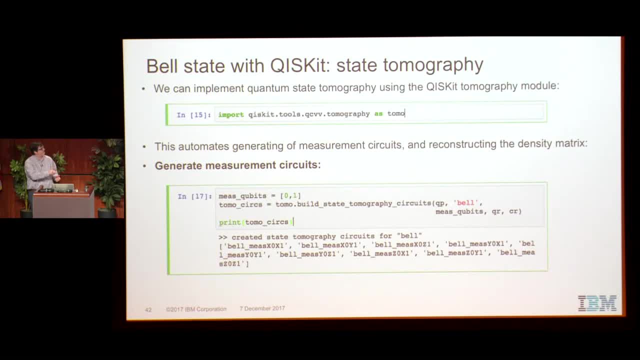 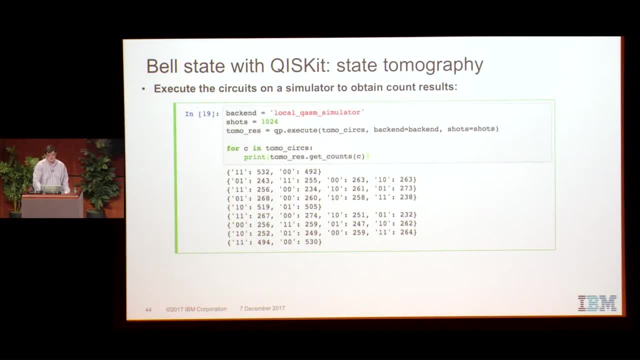 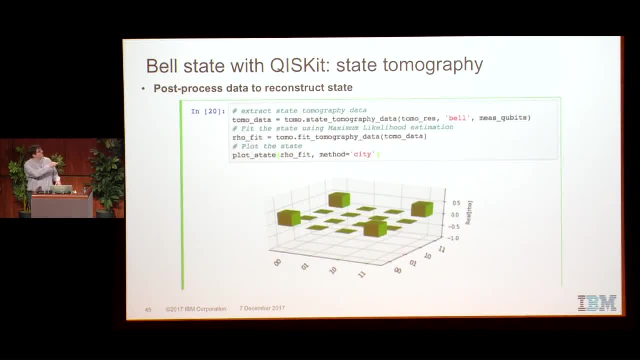 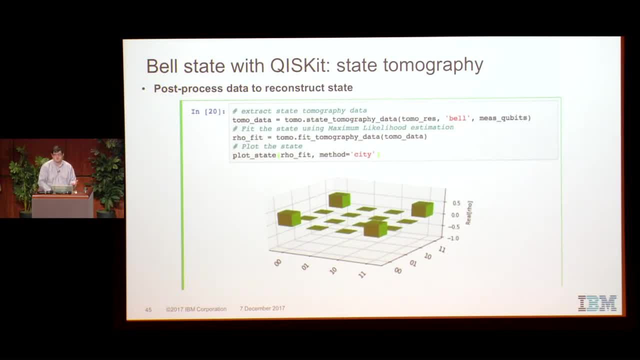 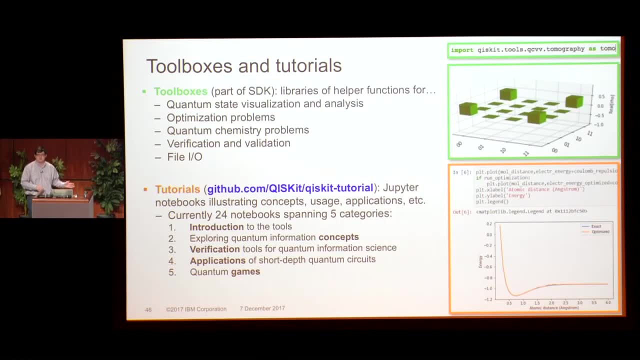 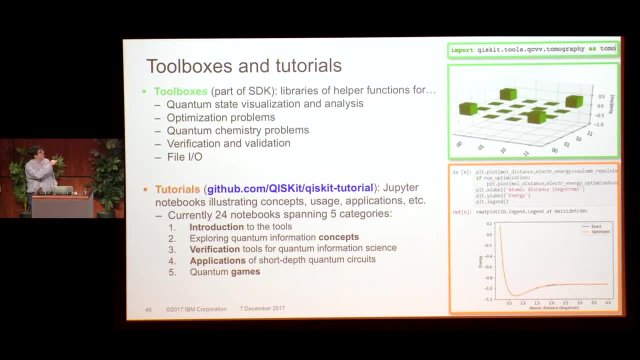 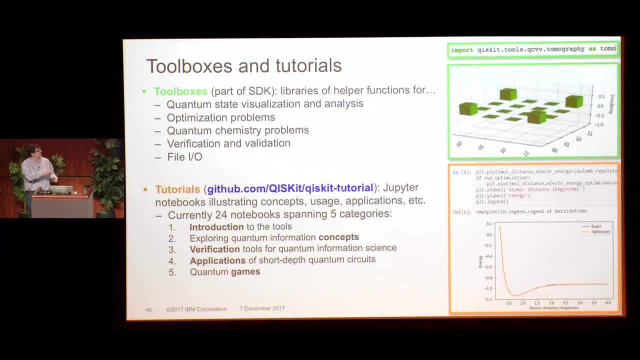 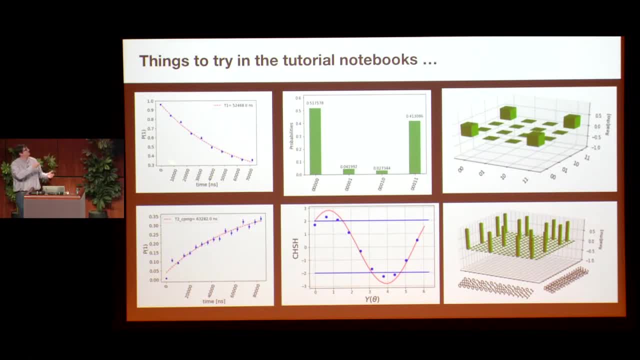 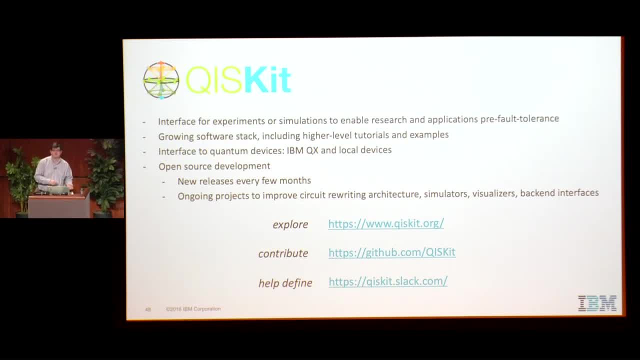 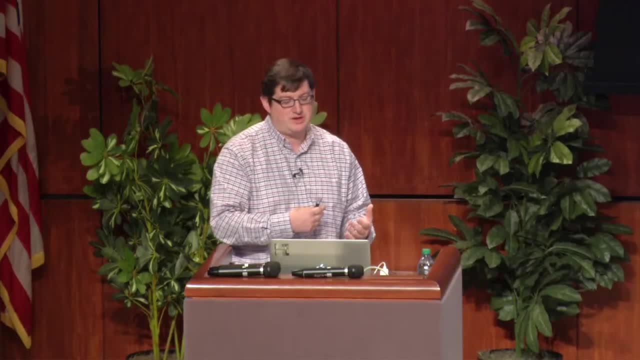 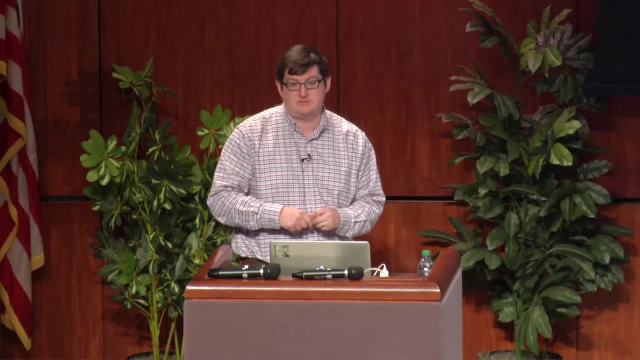 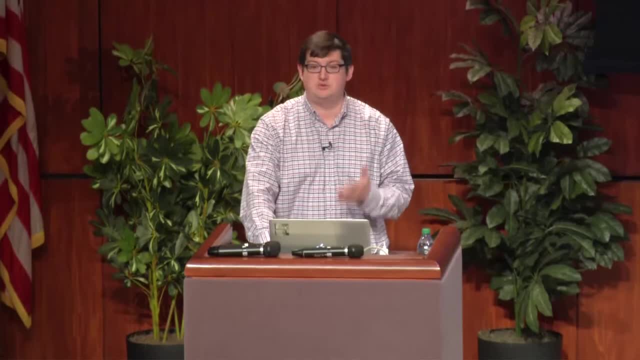 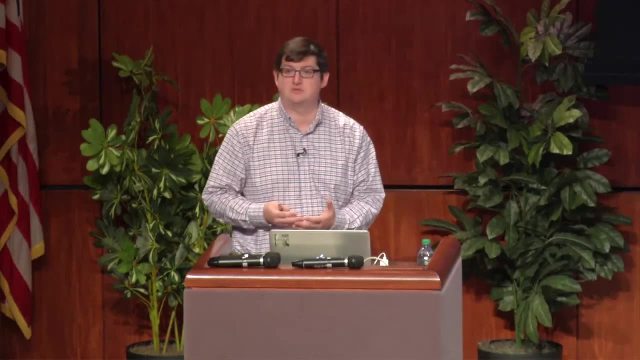 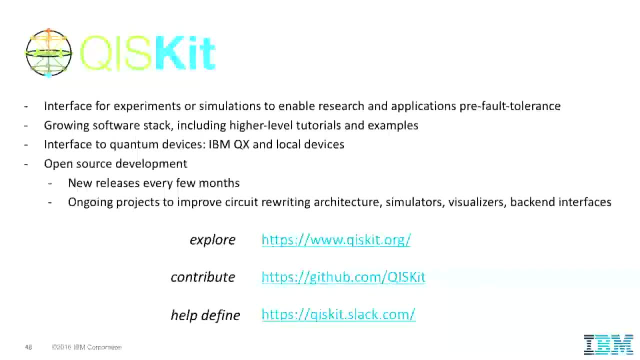